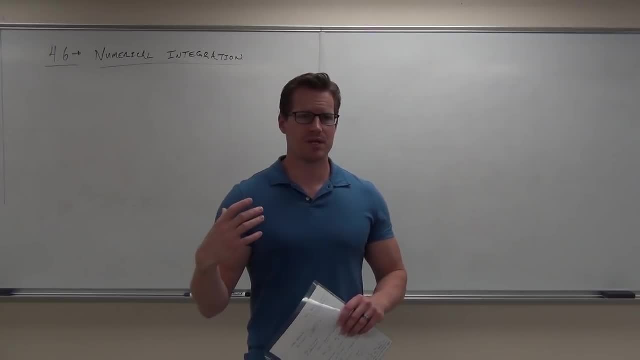 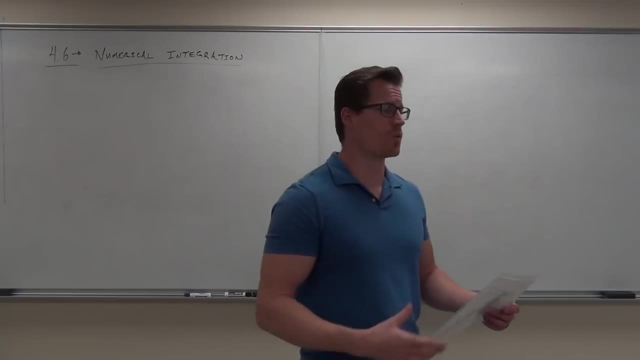 Okay, so the ones that we're going to do on the board. they would be something you'd learn in calculus too. Well, we've already learned them, But back then these integrals would have not been really possible for us, because we would not have learned them yet. 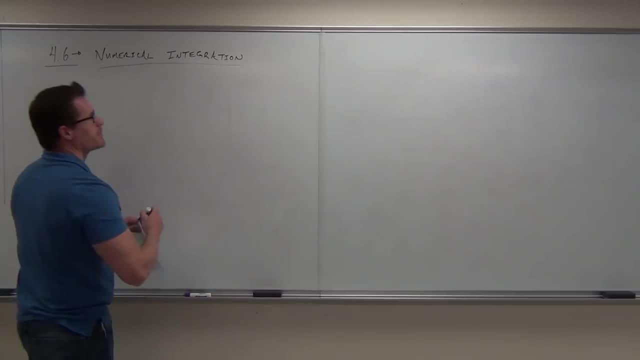 You with me? Okay. so with that in mind, let me introduce to you the trapezoidal rule. So the trapezoidal rule says this: If you want to approximate a definite integral, remember that definite integrals have bounds of integration. 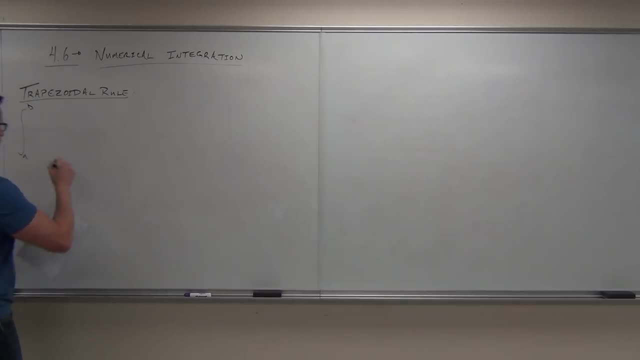 They go from like A to B. They go somewhere Of any function that you want. we can approximate it, Hence our squiggly equals here. We can approximate it by doing this, And it's really interesting. Here's how it works. 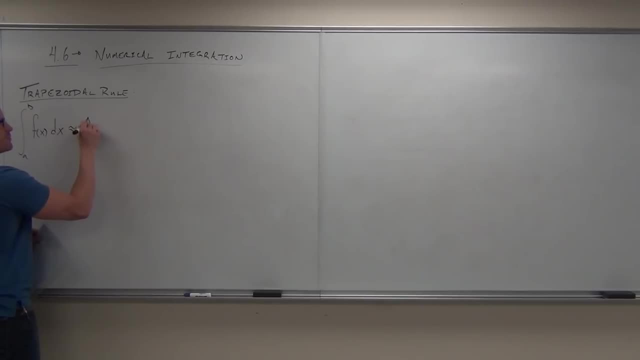 It says- and I'll define these in just a minute, but they should look familiar if you took calculus 1.. This looks familiar. Delta X. you guys have seen Delta X before, haven't you? We'll talk about that. I'll define it in a second if you don't remember what it is. 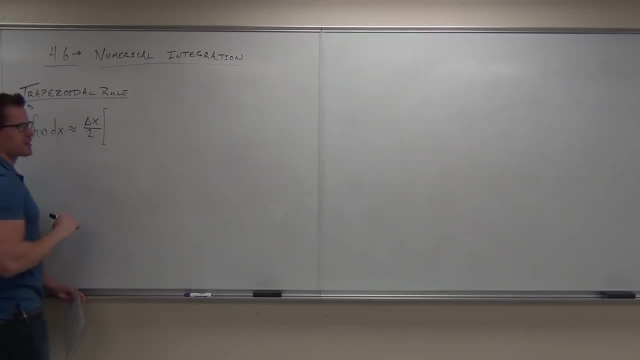 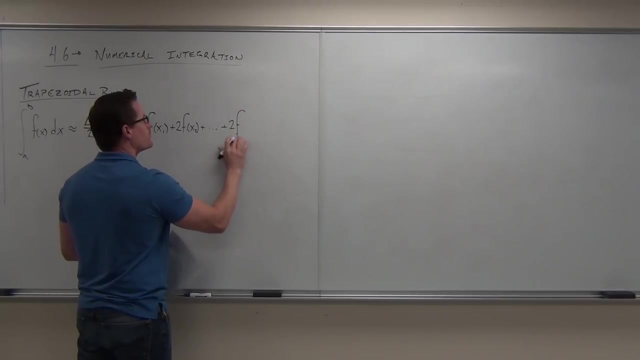 You take Delta X, you divide it by 2, and you multiply it by this sum By F of X sub 0 plus 2 times F of X sub 1.. Plus 2 times F of X sub 2 plus, and you keep all those 2s until you get down to 2 times F of X sub n minus 1 plus F of X sub n. 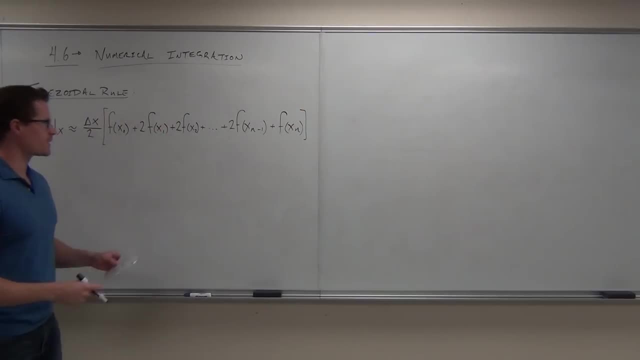 No 2.. That's the trapezoidal rule. Now I'm going to define a couple of these things for you. Firstly, what Delta X is. If you don't remember, And it's okay- Delta X is B minus A. 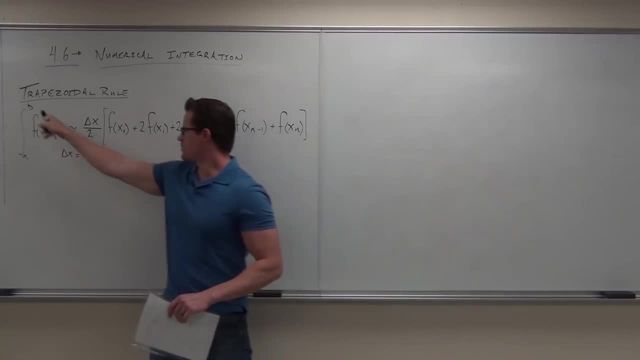 Where do I get my B minus A from, Do you know? Yeah, it's this here: B minus A. It's just your interval. So B minus A, divided by n, n is going to be given to you, So n is going to be some finite number. 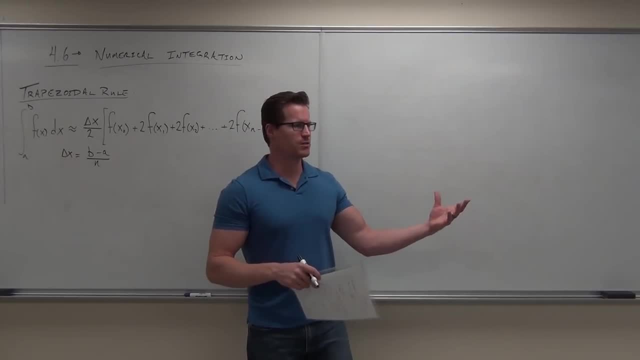 Because we're approximating right now. Now listen, We can't let n go to infinity, Because if we did well, we wouldn't have an approximation anymore, And this is going to. we wouldn't have a finite number of terms to add up. 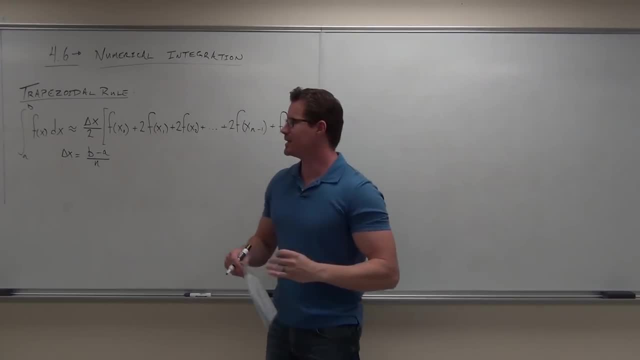 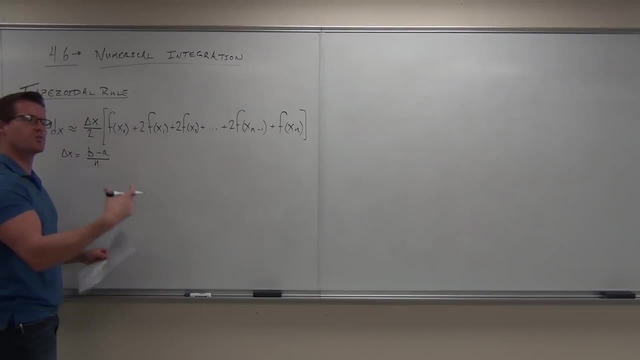 It wouldn't be an approximation. We can't actually do that. We couldn't do this forever. The idea of doing this forever Is the actual integrals that we've had. So if we could do the integral, well then we're left with a finite number of terms to approximate our value. 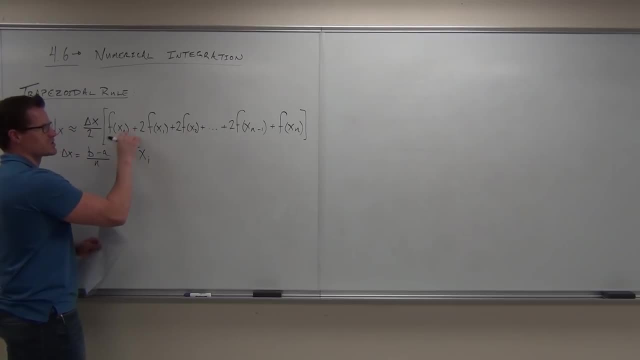 And then X sub I, Which means that X sub 0, X sub 1, X sub 2, X sub 3, X sub 4, X sub n minus 1, X sub n Is given by this. 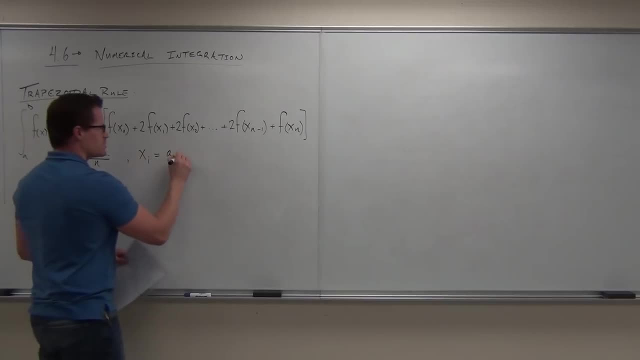 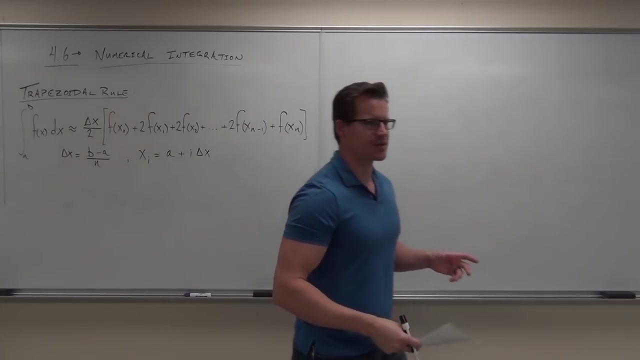 You start with A Again, A is just right here- And you add to it your index times, Delta X. That might look a little confusing. You've got to trust me on this. This is not that hard to do, And I'm going to prove that to you right now with an example. 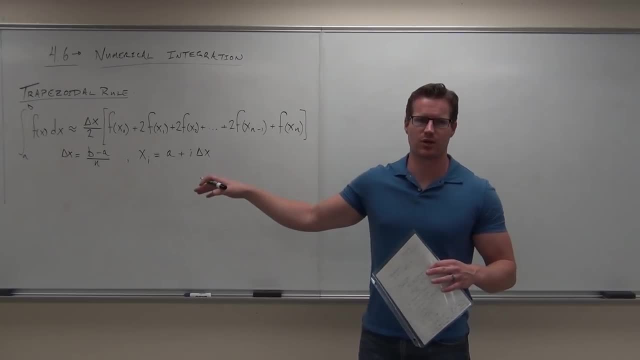 So write down the formula. I'm going to show you how to do it. Just make sure you write it down correctly. okay, There's no 2 in front of this. There's a 2 in front of every other term that you have, until you get to the very, very last one. 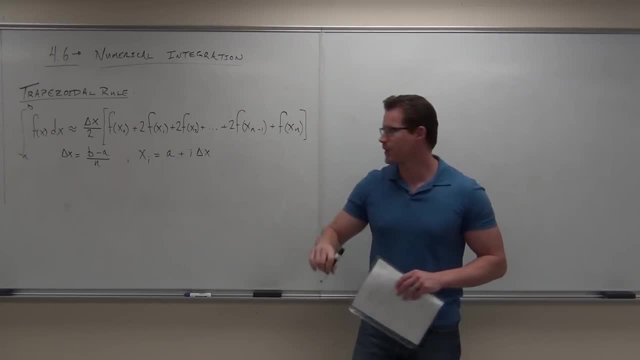 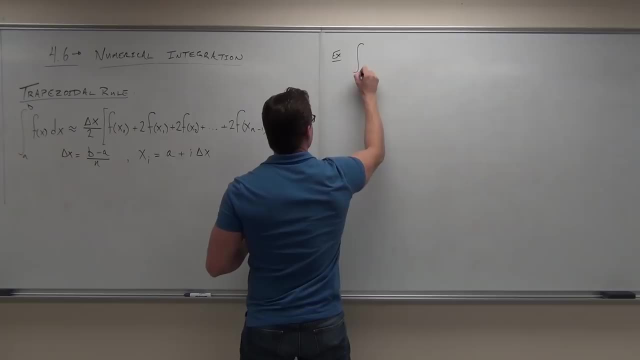 And then there's not a 2 there, Quick head up if you're okay with that. so far, Okay. So let's do our example. So what we're going to do is we're going to approximate 1 to 2.. 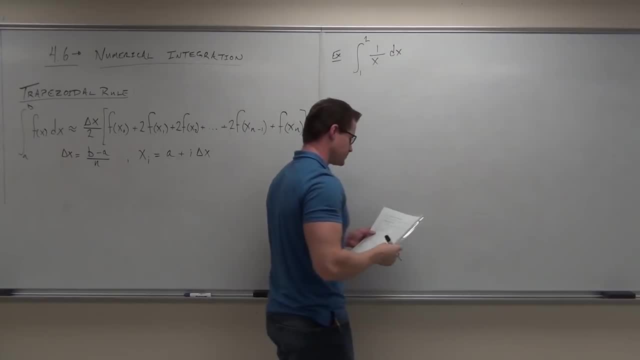 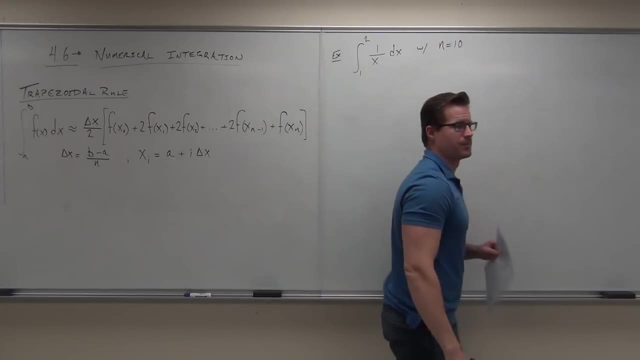 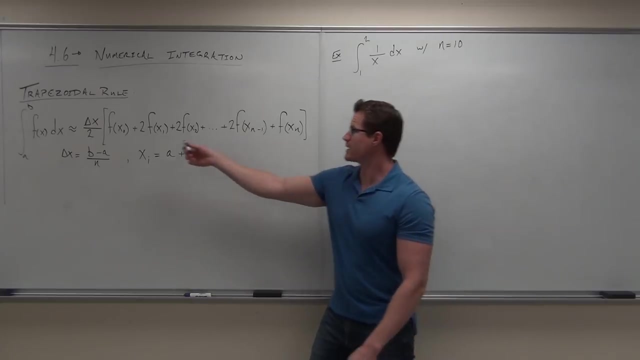 1 over X, And what we're going to do is approximate this with N equals 10.. If N equals 10, what that's going to mean for us is that we're going to get 11 terms here. We have an X sub 0 through X sub 10.. 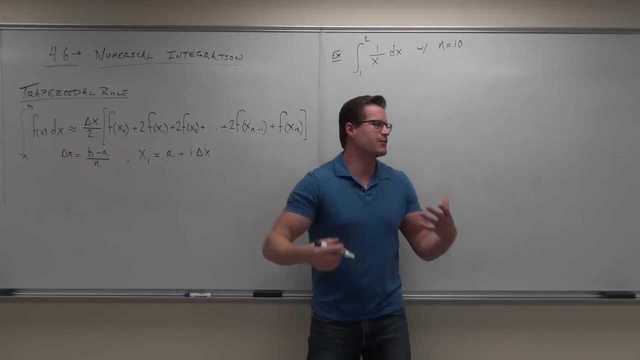 We're going to end on the X sub 10 term. Does that make sense to you? So we're going to get 11 terms. Stop at N equals 10.. Now, if you look at that, many of you are going to think: well, why don't we just do the integral? 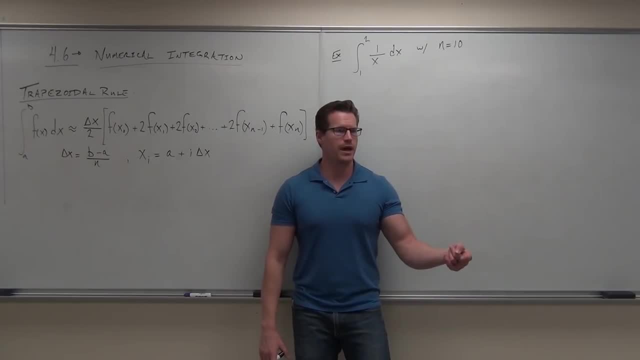 What's the integral of 1 over X? Would you know that in a late transcendentals class, like we have for Calculus 1?? Because in Calculus 1, we don't cover that. So that's why I said: put yourself back into Calculus 1,. first semester Calculus class. 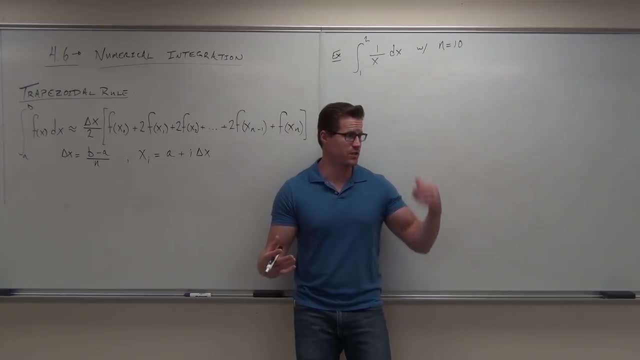 At our college we have what's called late transcendentals. Some people have early where they do this in Calculus 1. We don't, So we do it later. So for us this would have been impossible back in Calculus 1.. 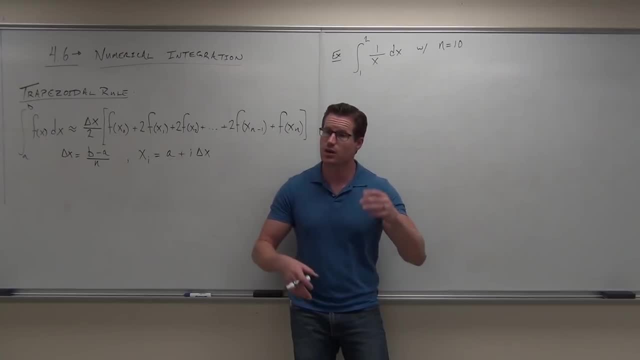 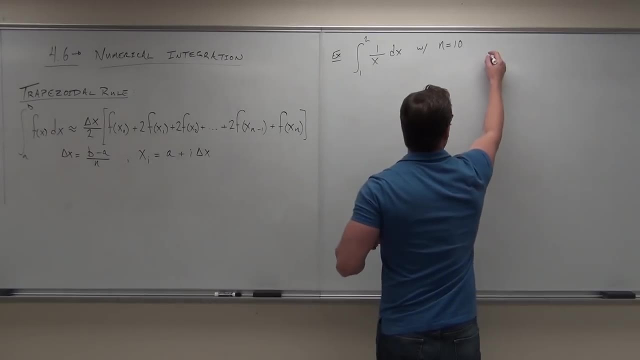 So all we would have done is try to approximate it. Here's how we're going to approximate it. The first thing we do, we figure out delta X. Of course that's going to be important for us. So to figure out delta X. delta X is B minus A over N. 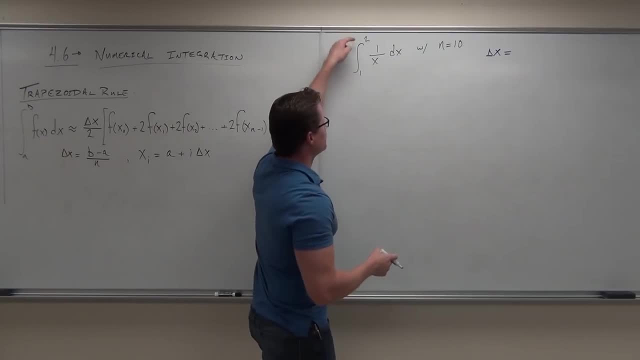 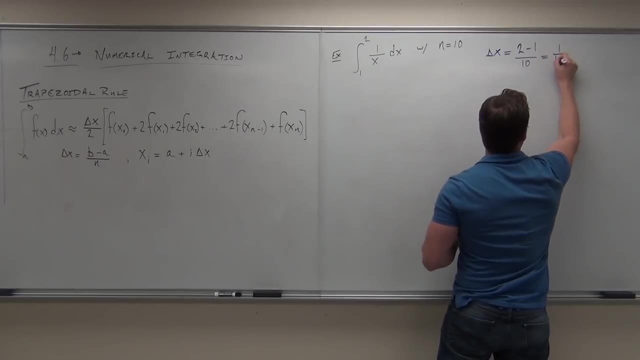 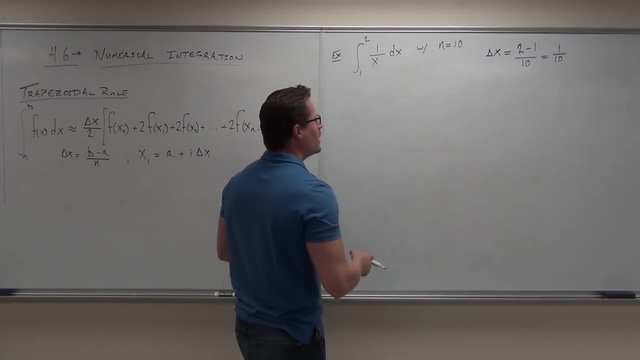 All those things are going to be given to you if you have a definite integral. What's our B Minus Over Perfect? That's going to be 110.. Okay, We're close to putting this in our formula. Now we've got to figure out our X sub 0.. 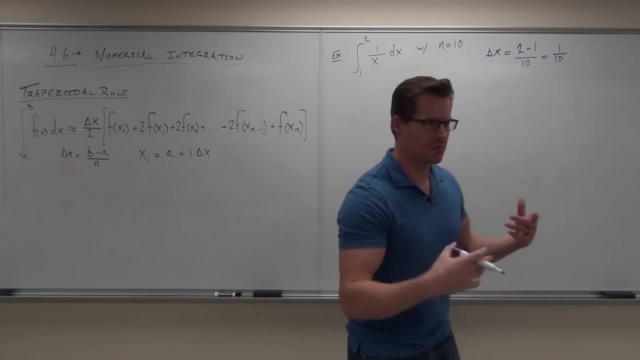 Our X sub 1,, our X sub 2, our X sub 3, our X sub 4, blah, blah, blah, blah, blah, blah blah. In fact, you can think of this as because we're going to be using calculators. 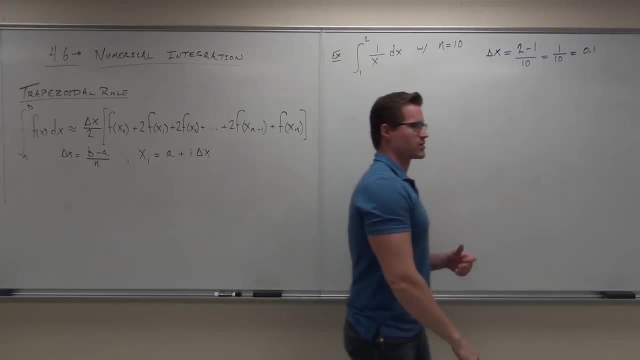 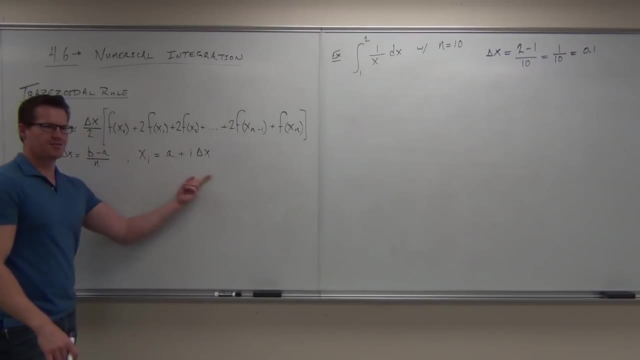 you can think of this as 0.1 if you want to. It might make things a little bit easier for you, if you want. So it looks kind of weird, Like how am I going to figure? It's not that hard. 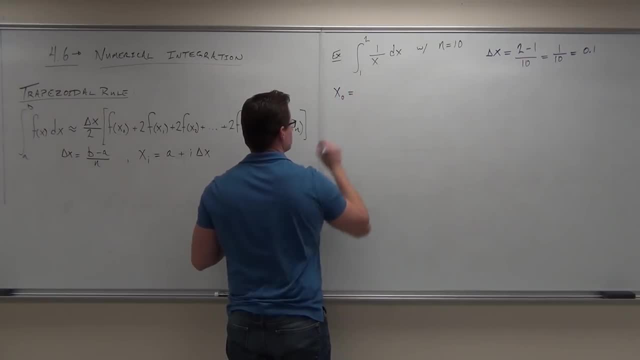 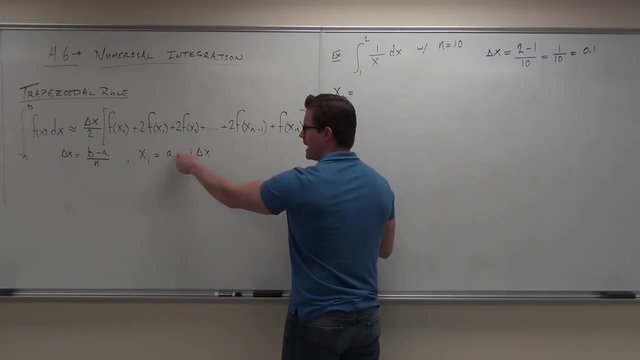 Here's what it says. If I want X sub 0,. X sub 0 says start at A. What's A? 1, 1.. Add 0 DXs, So we're just going to have 1.. Does that make sense? 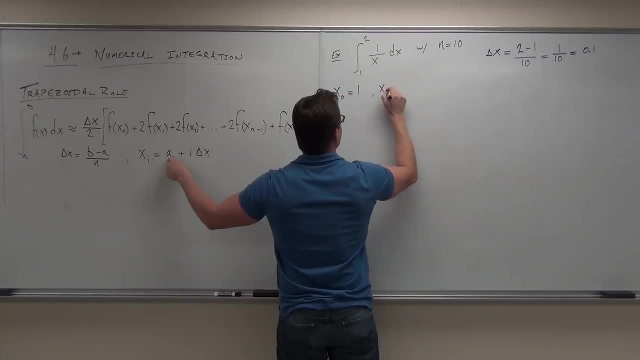 X sub. sorry, X sub 1.. I missed 1.. X sub 1 says this: Start at A, What's A again 1. And add 1 times delta X, So it would be 1 plus 0.1, or just 1.1.. 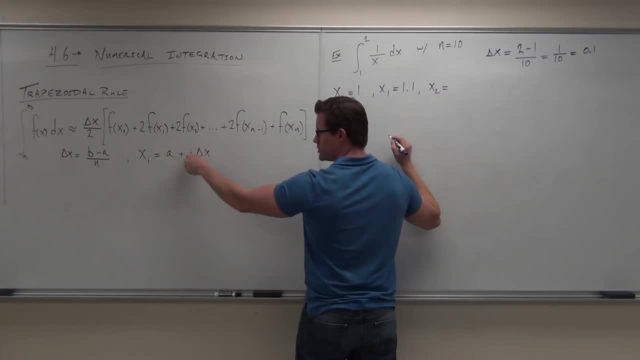 X sub 2 says start at A. It's 1 plus 2 times delta X. Well, that would be 1.1.. 1 plus 0.2, 1.2.. Can you tell me what the next one's going to be? 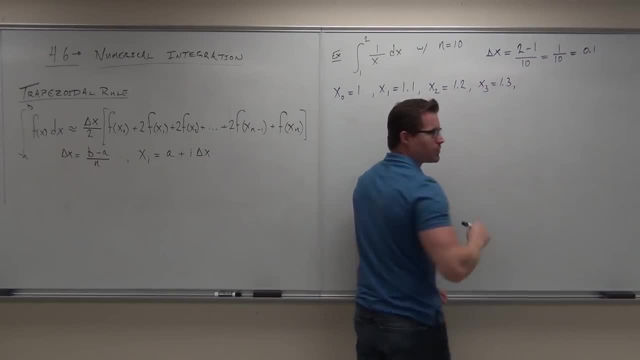 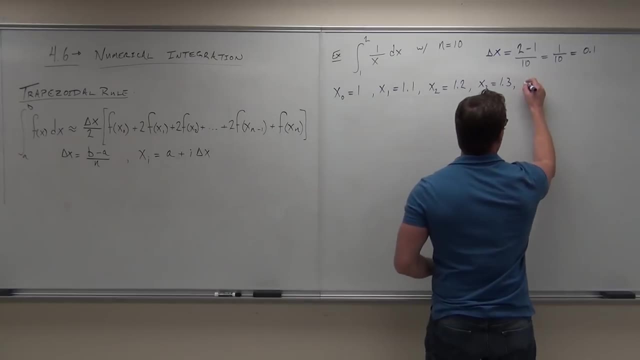 1.3.. What's the next one? And then 1.5, and then 1.6,, then 1.7,, then 1.8, and 1.9.. At the very end we're going to get to X sub 9.. 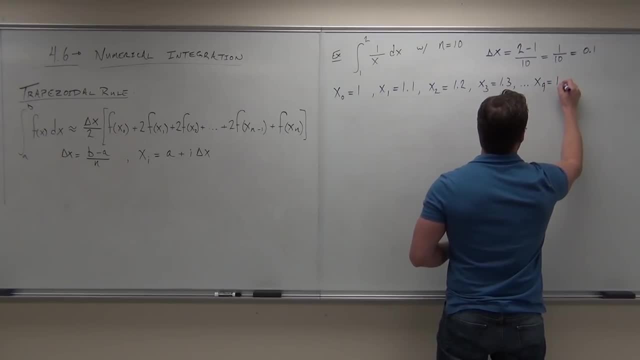 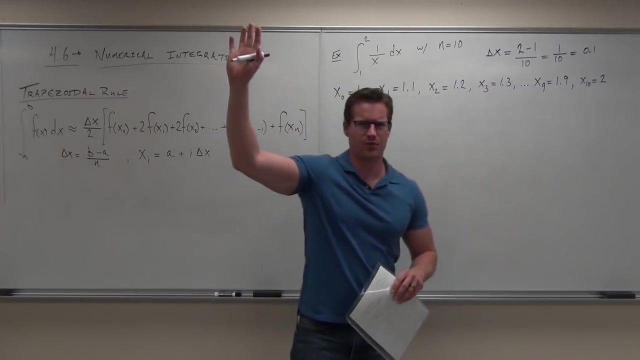 That's going to be 1.9.. And then X sub 10 gives you 2.. I want to show hands. if you're okay with where those are coming from, Can you follow that? It should be a little easier, because it's back to calculus 1 stuff. 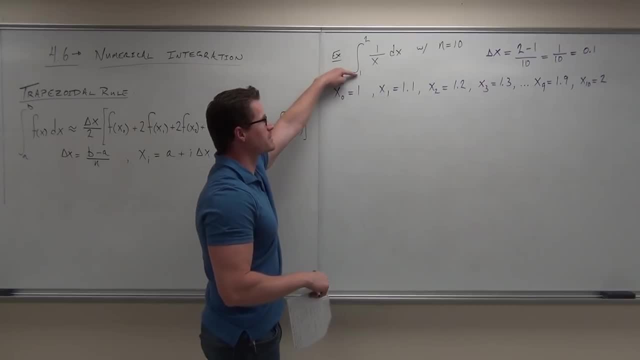 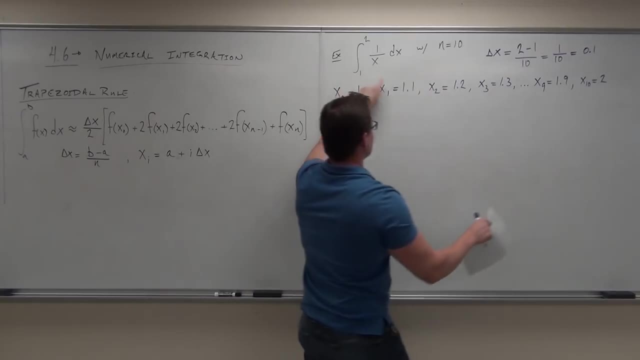 but just plug in numbers in It just says, hey, start here, start whatever that is, and just add delta X, So for X sub 0, you add none of them, So it's just 1.. And then add this: 1.1.. 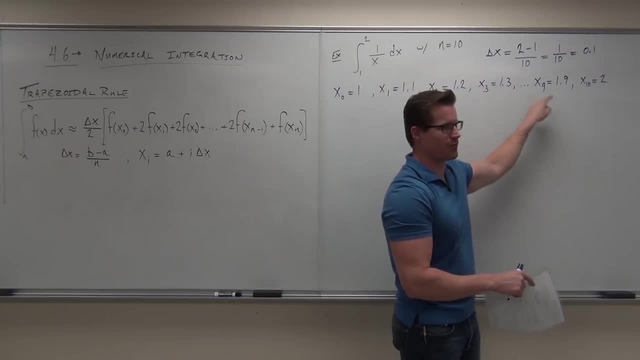 Add it again: 1.2.. Add it again 1.3,, 1.4,, 1.5,, 1.6,, 1.7,, 1.8,, 1.9, and then 2.1.. 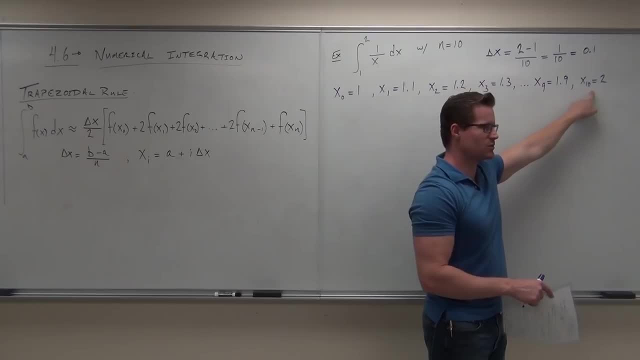 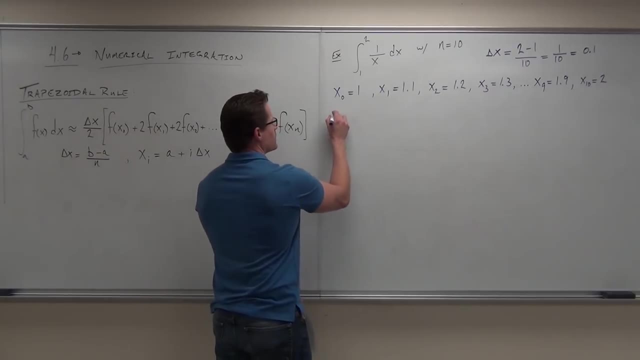 1.10, 2.. Yeah, so we get 2.. Now what the trapezoidal rule says is: after you've done all that, the integral can be approximated by doing this. You take delta X. What's our delta X? 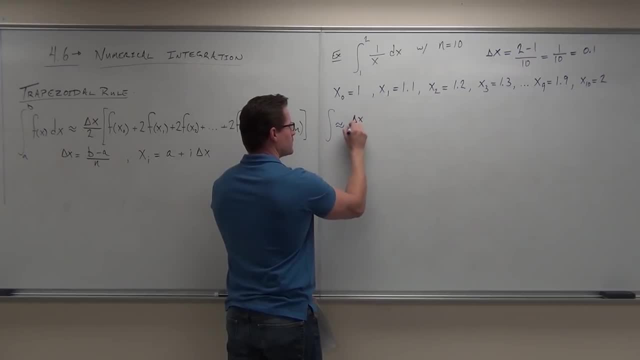 1.- 1.. So we have delta X over 2.. And then you're going to do this, You're going to have F of X sub 2. Zero F of what Plus? what's the next thing I'm going to write? 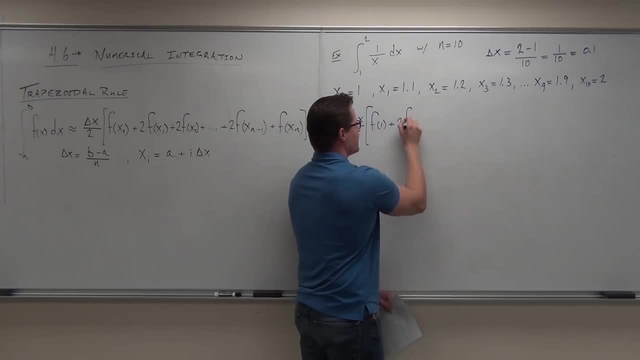 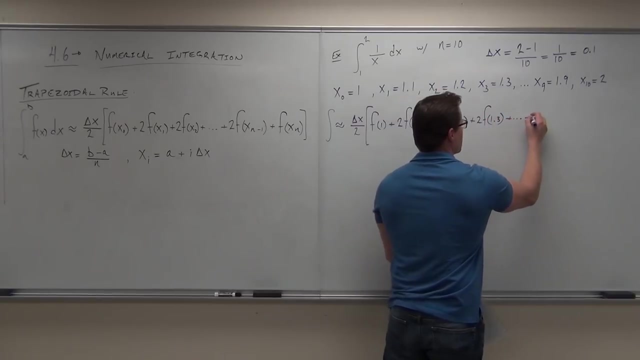 Now our 2's start: 2 times F of what, Yeah, Plus 2 times 1.2.. Plus 2 times F of 1.3.. Plus we're going to do this all the way down until we get to 2 times F of 1.9.. 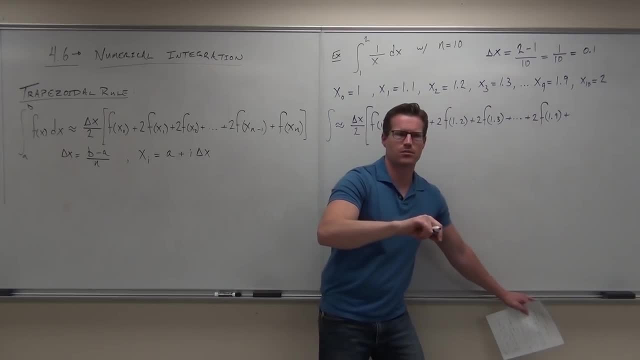 And then we're going to do this all the way down until we get to 2 times F of 1.9. And then we're going to have: do we have a 2 on the very last term? No, No, It's just F of 2.. 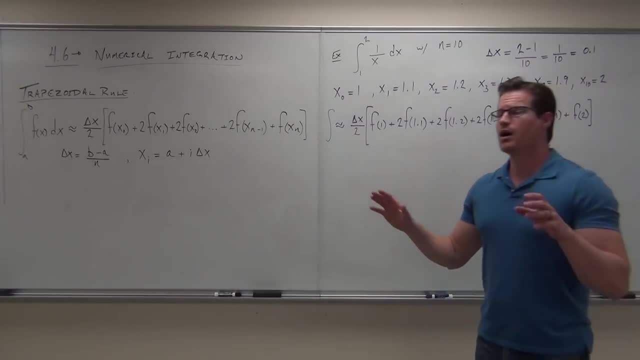 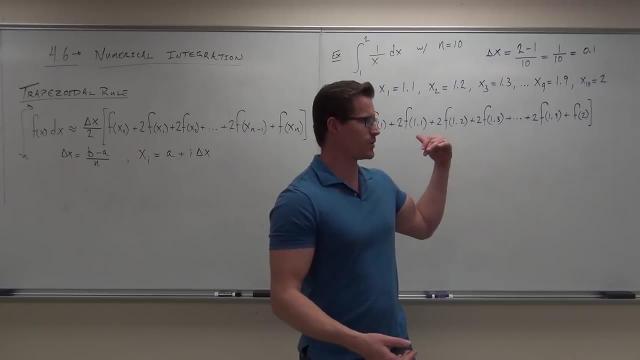 Okay, I want to do like a 20-second recap, just to make sure that you get this. So the idea behind these numerical integrations is: sometimes we can't integrate or sometimes we don't know how to integrate it, And this would be one of those cases where, at the time, we would not have known how to do this. 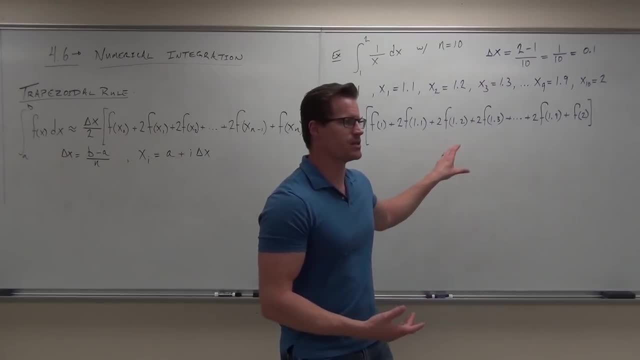 Now I'm giving you a very simple example. okay, Just so. it makes our math easy. so you get the idea. You could do this with some pretty hardcore integrals that you don't know how to integrate If it's a definite integral. 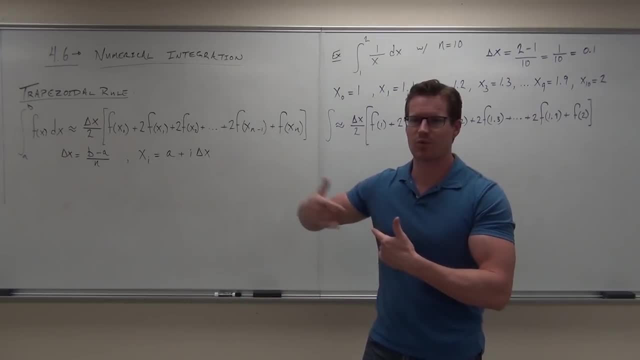 Do you understand that if it's not a definite integral, this doesn't work, Because I'm plugging numbers in. all right, So what we say is all right. where's your integral starting, Whatever, Where's it stopping? 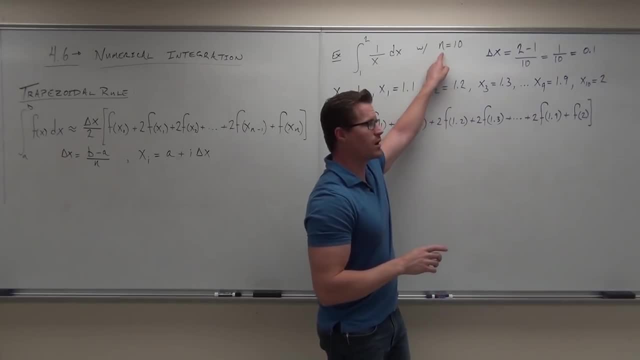 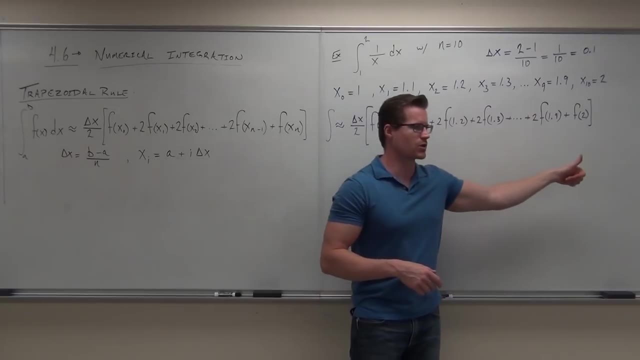 Whatever You can find delta X with that, provided you're given the number of iterations in your rule. So in this case we have N equals 10. That's 11 terms that we're going to be going through. So it says: okay, cool. 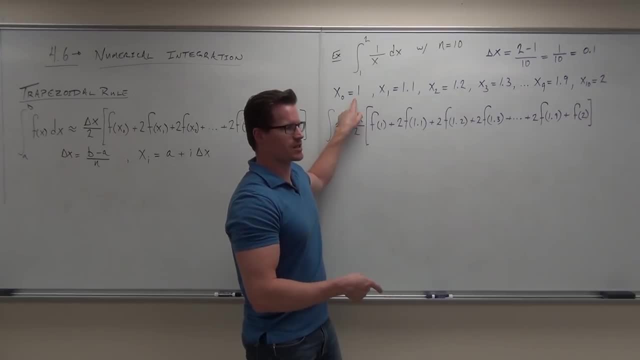 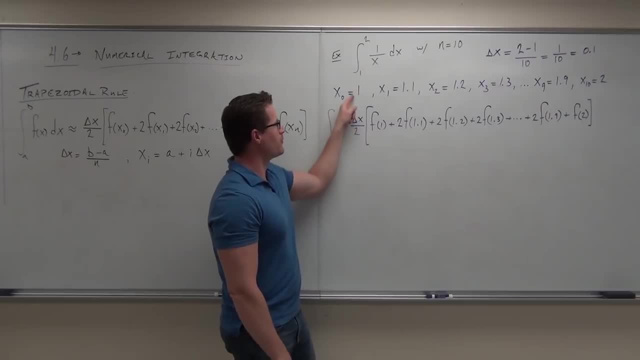 Plug in the formula. We have delta X over 2,, no problem. F of X of 0.. F of X of 1.. So 1 and 1.1, 1.2, all the way to the very end. 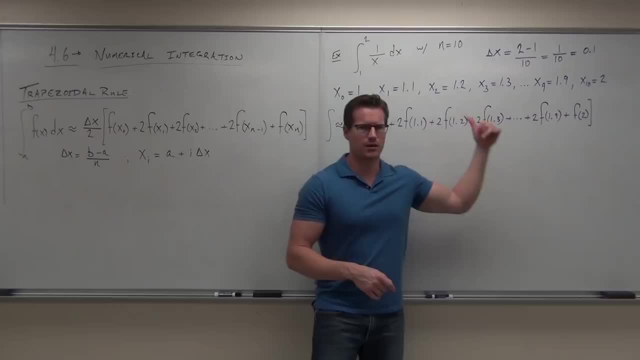 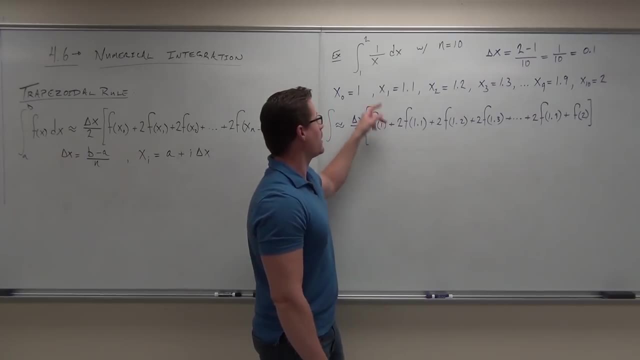 Notice, the only two terms that don't have 2's are the first one and the last one. You follow. Now, what's nice about this? do you have a function that you can plug these things into? Yeah, it's right there. 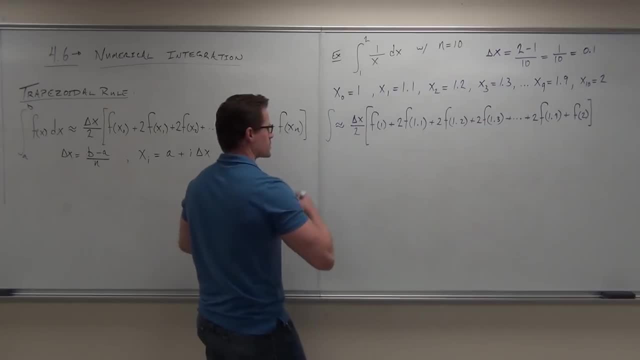 It's just 1 over 2.. It's 1 over X. So we're going to do this. We're going to start by taking our delta X. It's 0.1 divided by 2, and then we're going to have F of 1.. 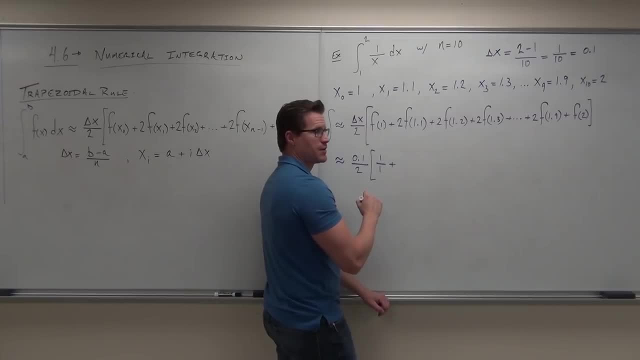 So that's 1 over 1 plus 2 times F of 2.. So check it out: It's going to be 2 times 1 over 1.1 plus 2 times 1 over 1.2 plus 2 times. 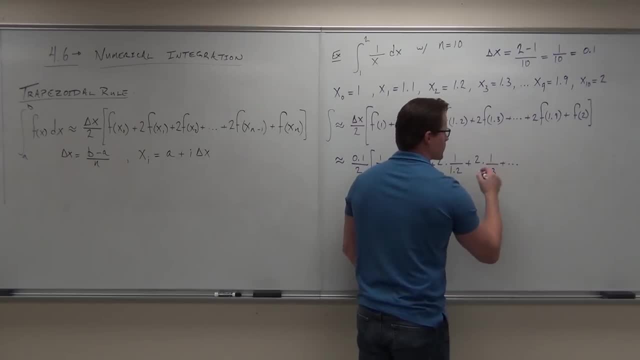 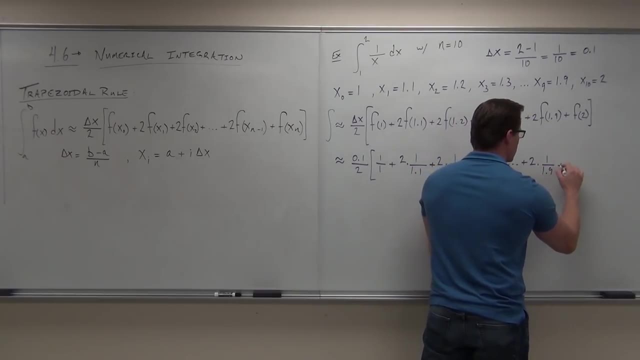 1 over 1.3 plus we're going to do this for a while, for a finite number of terms, and we're going to end off with 2 times 1 over 1.9, plus 1 over 2.. 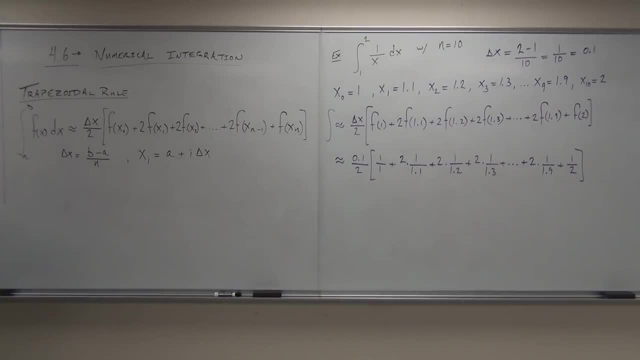 I want you to see if you can go through that in your mind, if that actually makes sense to you. Show of hands. if that does make sense to you, Okay. so here's what you're going to do on your calculators. What you're going to do is you're going to figure out what all these things are. 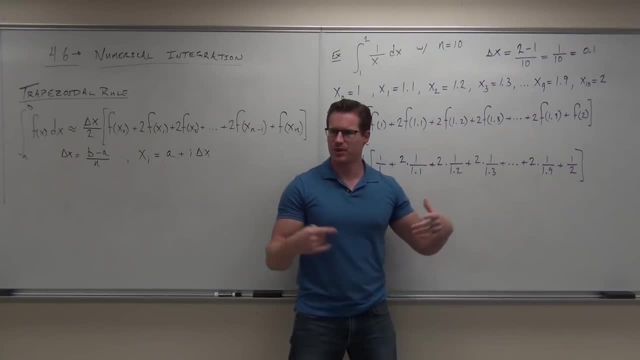 I'm not writing all of them because it just takes too long, but I'm hoping that I've made this clear on what this is. Do you guys see what it is? We start off with just a function evaluated at whatever. our A is just 1,. 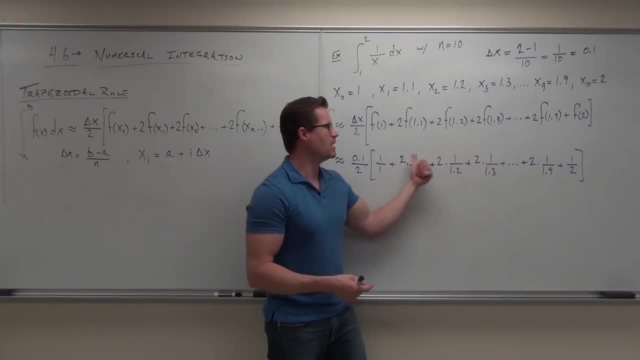 and then we add to it 2 times F of 1.1, 2 times F of 1.2, 2 times F of whatever, our X of 3, our X of 4, our X of 5, all the way up until we get to our X of N minus 1.. 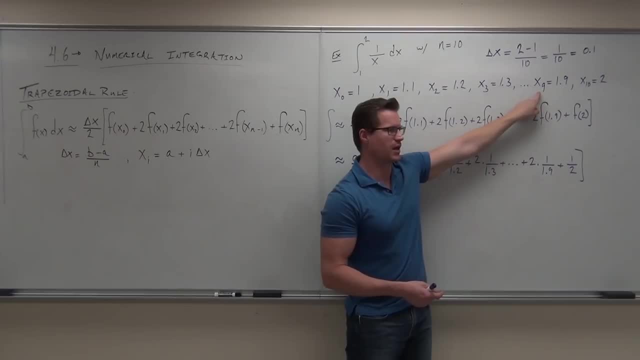 Look at that. X of N minus 1 is 9.. Some of you guys on your test did X of N plus 1 for this one. You were counting further than you should have been counting before, not after. So X of N minus 1 gives us our 9, and then our last one, whatever it is, in 10 in this case. 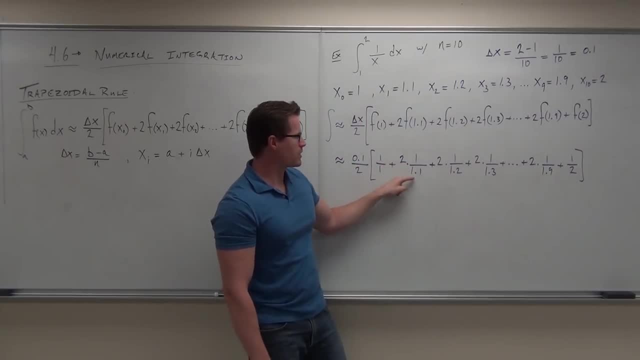 No 2 here. We plug them into our function. That's why we have our 1 over this, 1 over this, 1 over X of 3,, 1 over X of 10, and we just figure it out decimal equivalent. 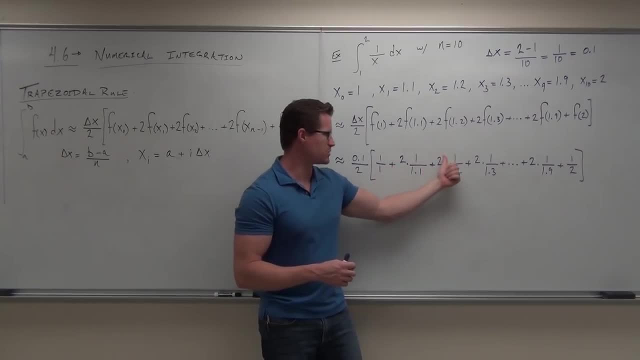 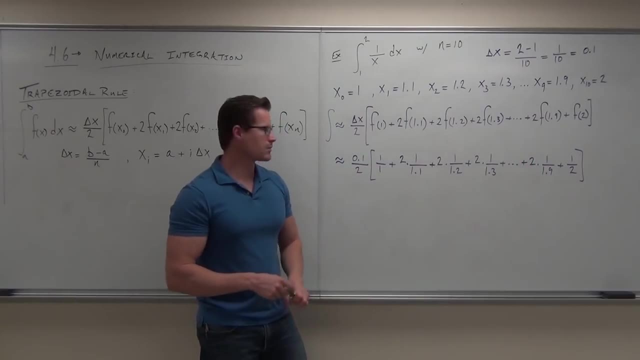 So, in our case, on your calculator, you get 1 plus 2 over this, plus 2 over this, plus 2 over that, blah, blah, blah, and then multiply that by 120.. Now, as you're doing that, I'm going to go ahead, I'm going to. actually, I did this on purpose. 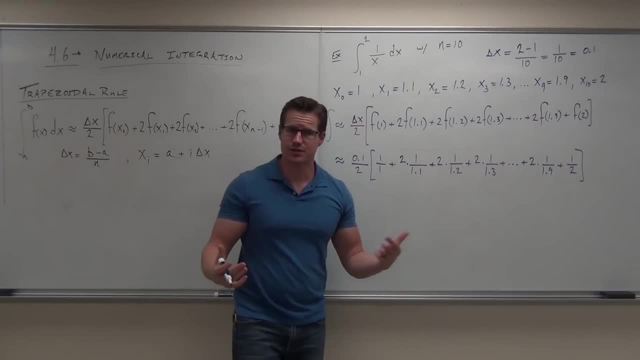 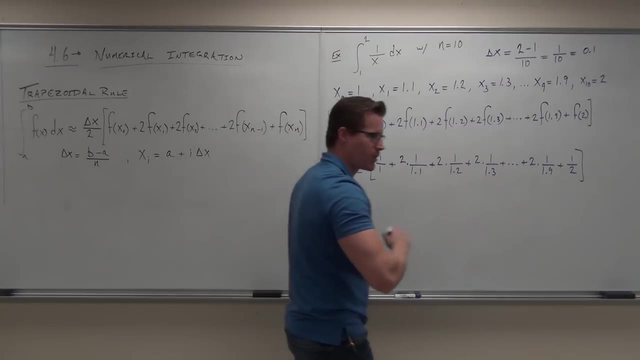 I did the integral because we can actually do it. I wanted to see how close this actually is, So if we were to really do the integral. so keep on working on this. Some of you guys really go through this. okay, I want an actual answer. 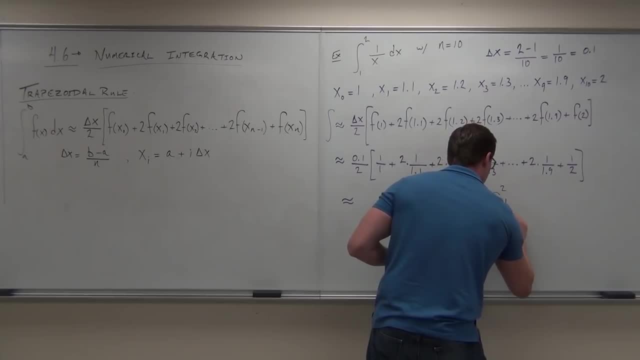 So but if we were to do the integral with what we know now, we know the integral of 1 over X is LNX, right LNX, and we would evaluate that from 1 to 2.. That's LN of 2 minus LN of 1.. 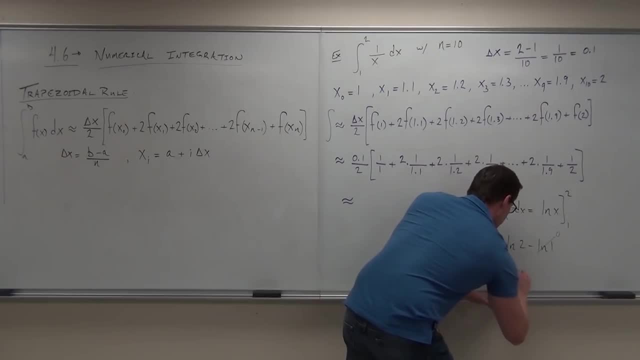 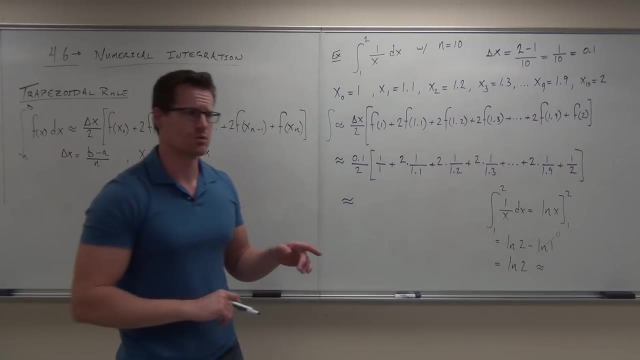 Well, LN of 1 is 0, so we'd get LN of 2, and LN of 2 is about equal to someone who's not working on this. can you tell me what LN of 2 is about equal to? 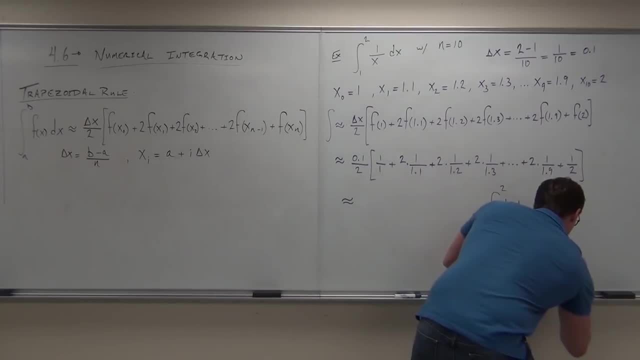 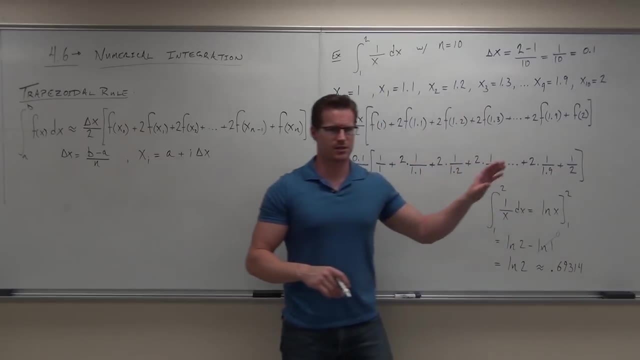 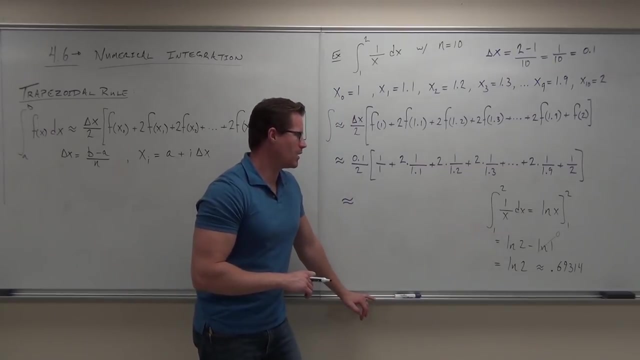 0.69314.. 0.69, say it again: 69314.. Okay About that. it keeps on going Because it's well, it's an irrational number. It goes on forever without ever repeating. Have you got this one? 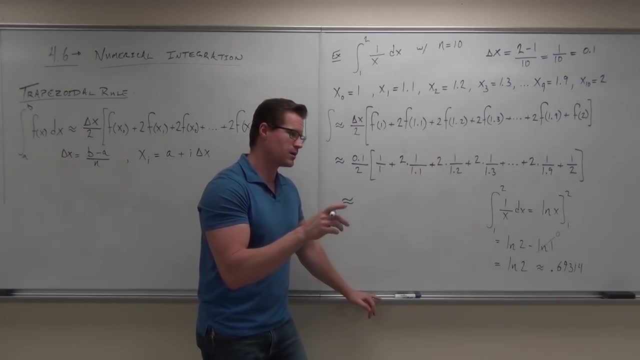 Yeah, What'd you get? 0.69377.. Yeah, okay, Is it exactly the same? No, but it's close. Is it close? No, Tenths, hundredths, it's the same to the thousandths. 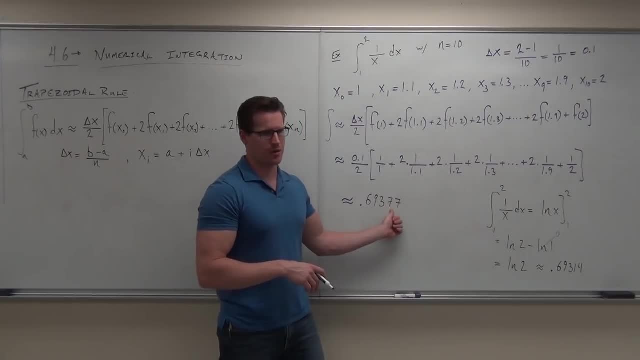 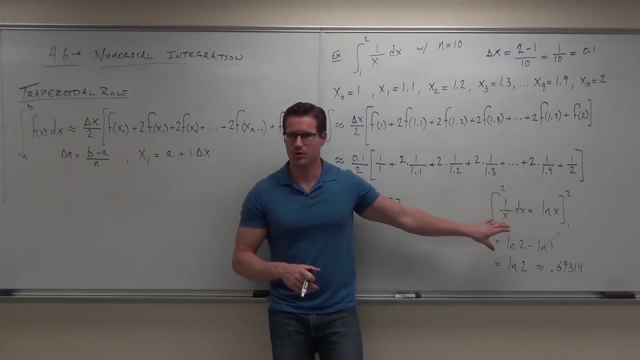 It's off by a little over 6.. It's 10 thousandths so with if you. but here's the point: This was quicker because we know how to do it right. If this was an integral that we didn't know how to do, this would be the best way. 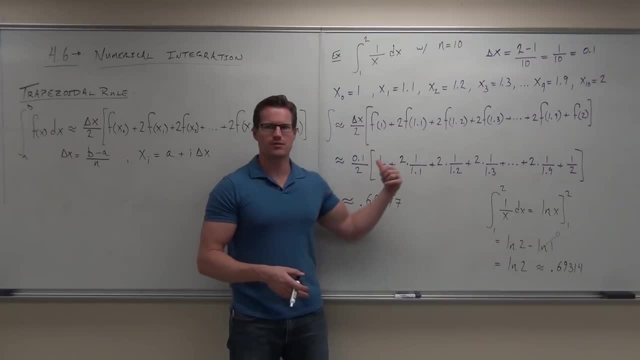 because you don't know how to do it. So you go, okay, well, cool, Let's evaluate this approximately, Let's use our trapezoidal rule, and then we get something that's relatively close. Now question: how do you make this better? 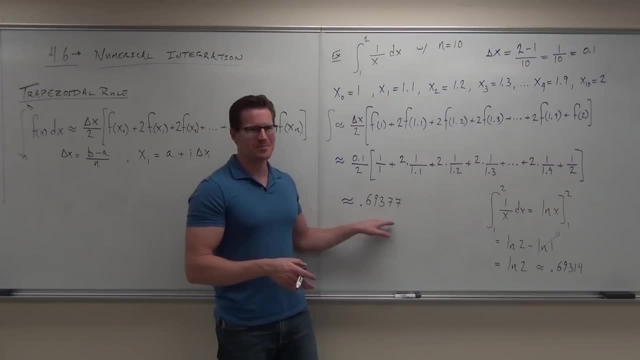 Plus C, More terms, Not plus C, because it's definitely an integral. How do you make it better? Yeah, Yeah, Yeah, Yeah. How do you make it better? More N, More Ns, Do that to like 100.. 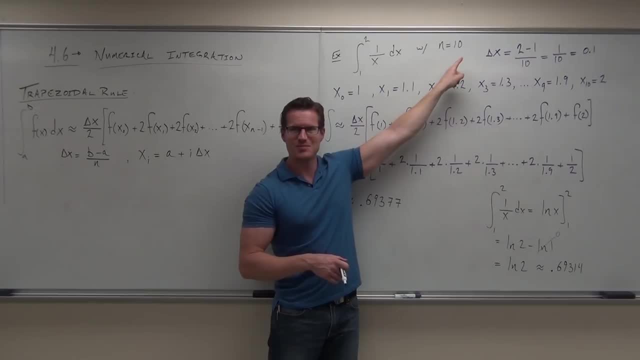 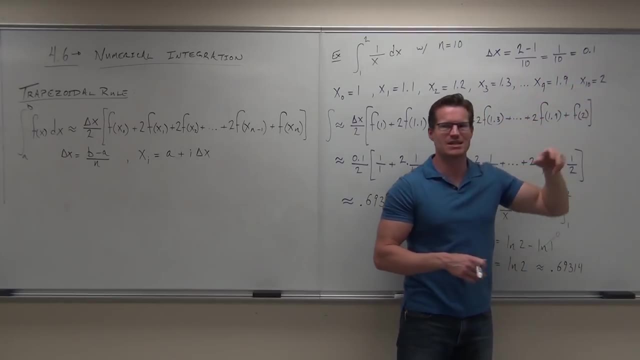 It's really close, Annoying. It's very annoying, but really close, because what's happening is you're taking our interval and you're making it really, really, really little. It's the same idea with doing Riemann sums with more N, with N equals larger numbers. 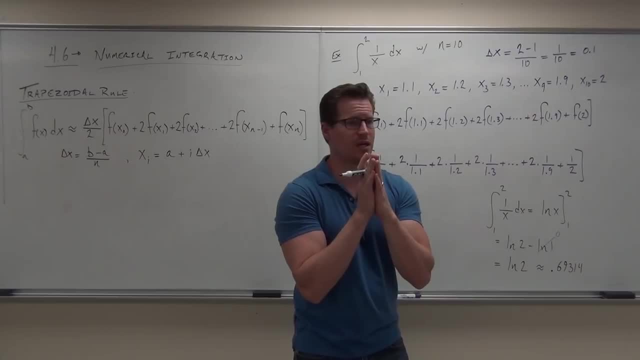 You're making smaller rectangles, Smaller rectangles. well, hey, if you have smaller rectangles, that means you're missing less and less area when you add up those rectangles. If you remember back to your, Your Riemann sums that you did count this one. 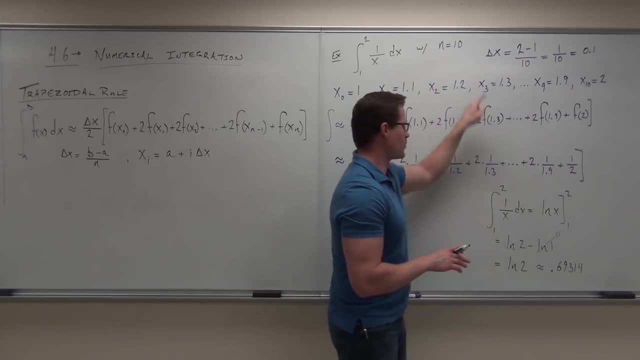 Is that making sense to you? So the bigger that is, the more close this is going to be. I just want to do this one to show you, hey, you know what. You can actually approximate it and get it pretty darn close. 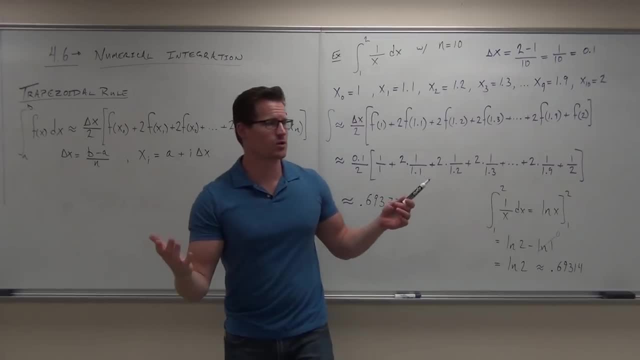 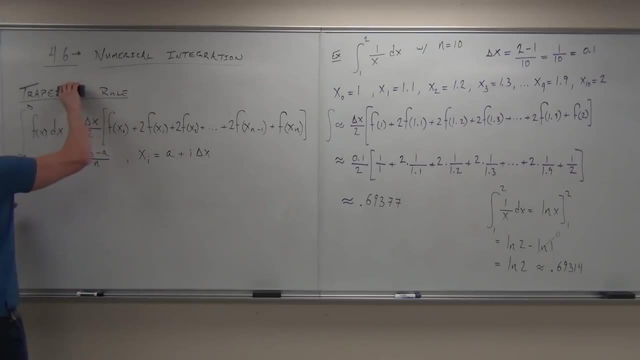 Show your fans if I explained that well enough for you. Okay, This is it for trapezoidal rule. That's how it works. I'm going to give you Simpson's rule. I'll show you how Simpson's rule differs. Here's how Simpson's rule works. 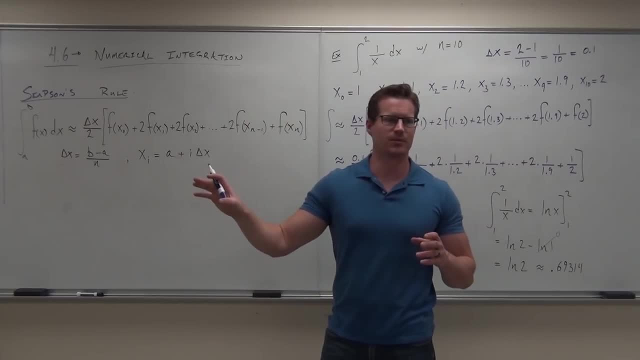 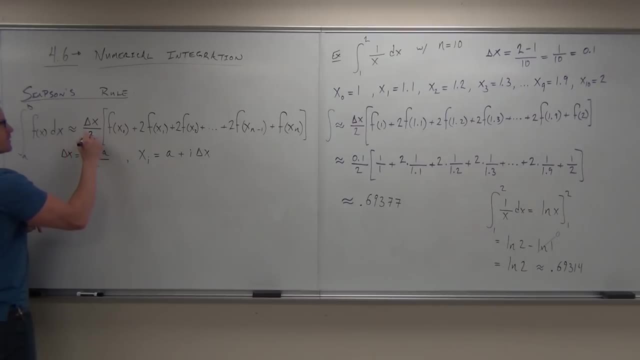 Simpson's rule is going to look really, really similar. Here's the only difference: Instead of taking delta X divided by 2, you're going to take delta X, you're going to divide by 3.. Then what you do? Yeah, I know right. 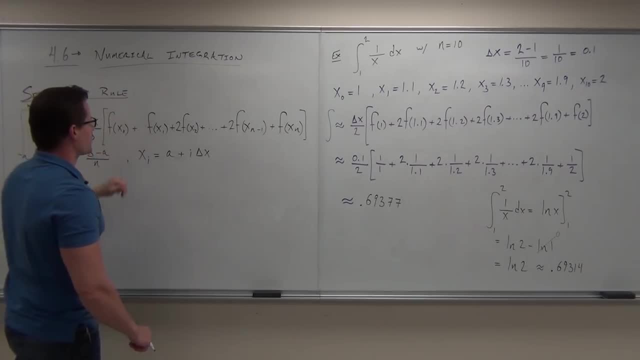 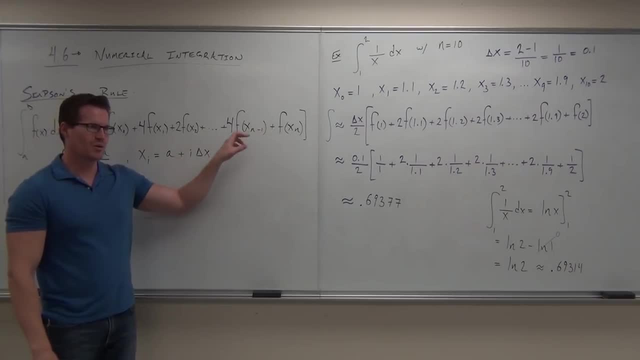 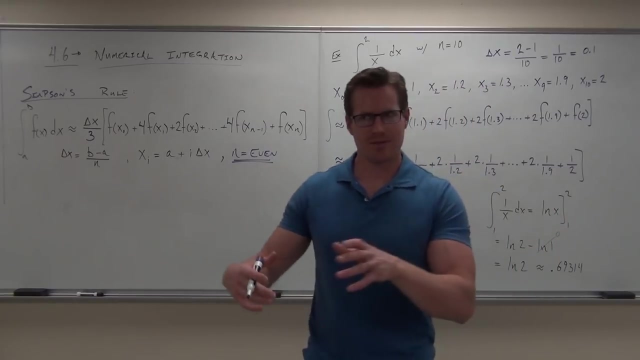 And then that last one doesn't get anything. Now, this will only work if N is even. N's got to be even. So you can't do this if N is 5.. You could do it if N is 6, or if N is 8, or 2, or like what even numbers are. 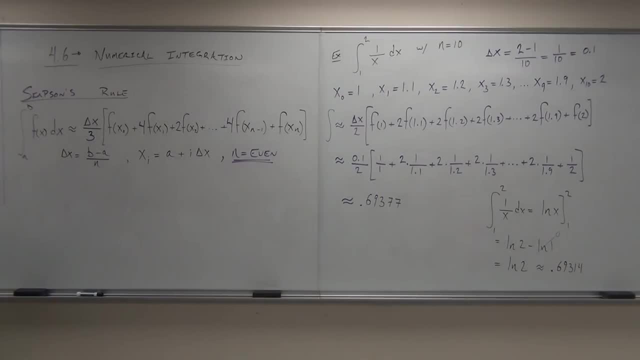 You do it evens, but other than that, this won't work for you. Make sure I wrote it down right too. I did it from memory, but yeah, I think I got it. You guys want to do an example here real quick. 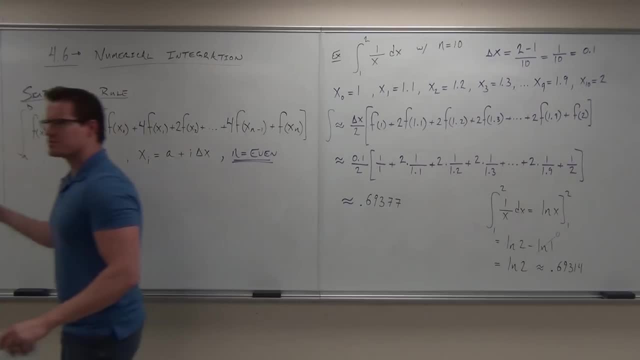 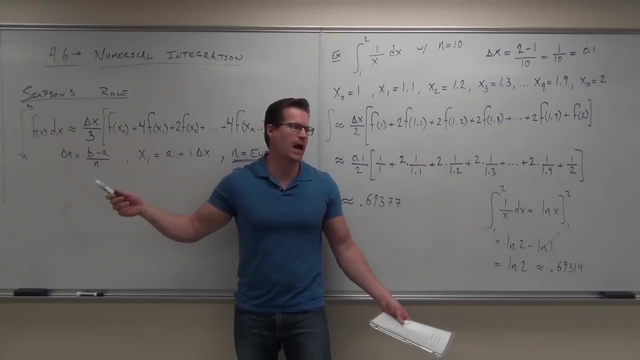 Yes, please, Okay, Does this make sense to you that we're going to alternate 4s and 2s? Just, you don't end with a 2, you end with a 4.. That's going to happen if you have an, even okay. 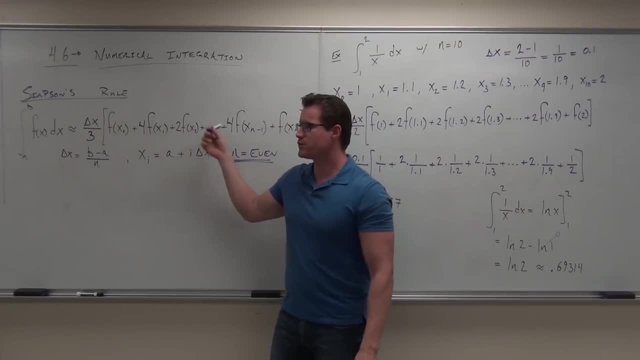 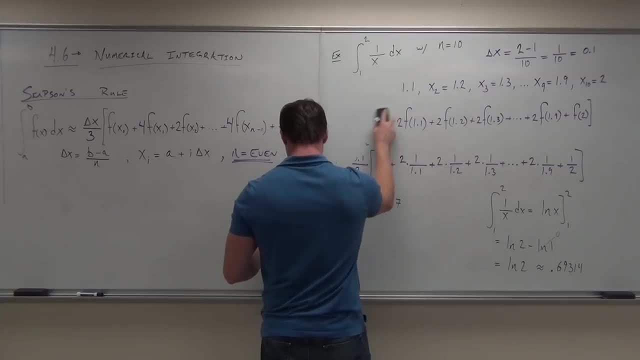 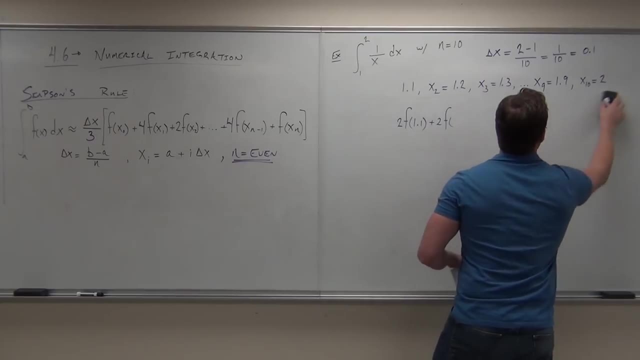 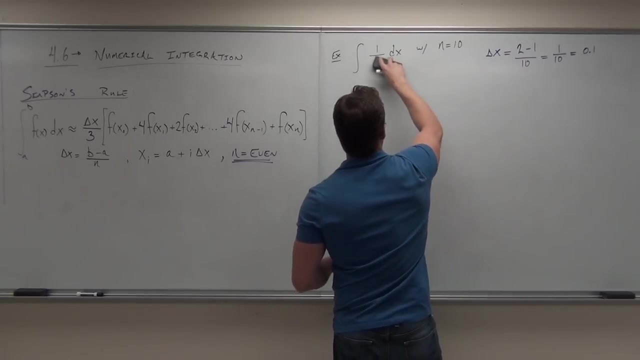 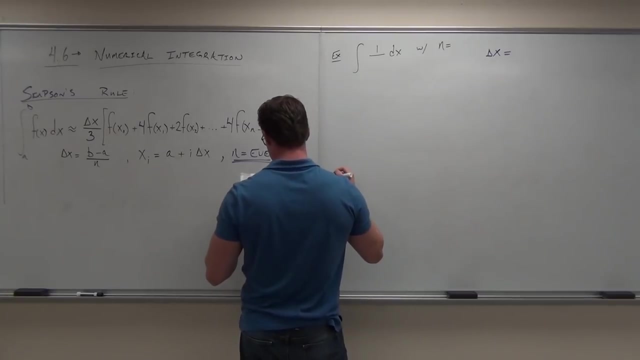 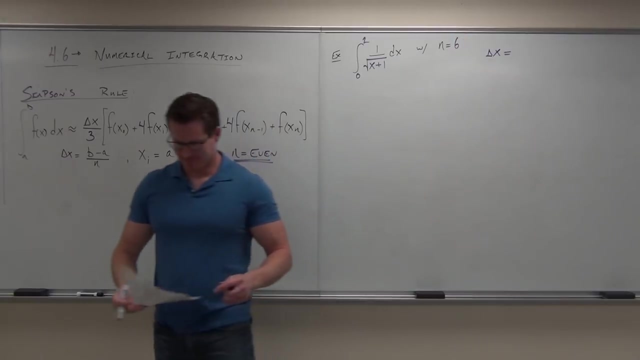 So let me change this just a little bit. How about 1 over square root x plus 1 from 0 to 2, with N equals 7? Is that okay? No, Why not? It has to be even Okay. fine, you sticklers 6,, N equals 6.. 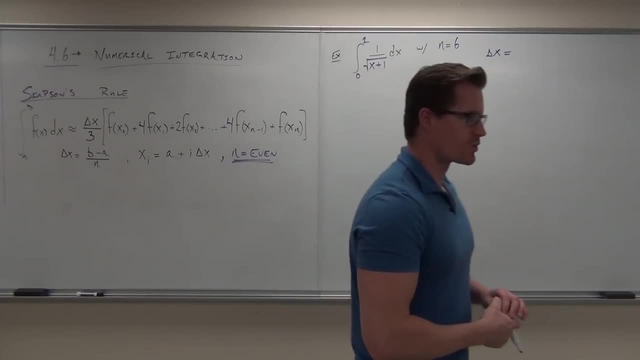 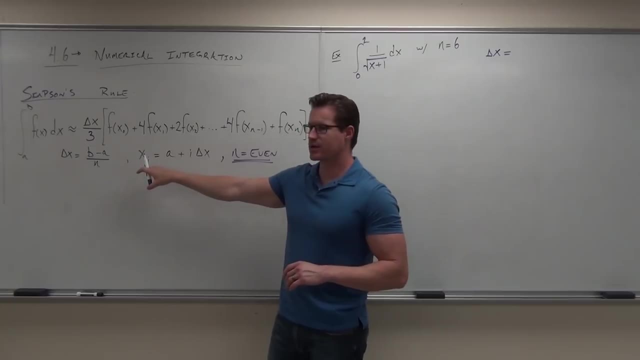 Go through the same way that you would normally do the trapezoidal rule. only now we're just going to plug it into a different formula. The delta x is calculated the same way, The x of i's are calculated the same way, and it just has. 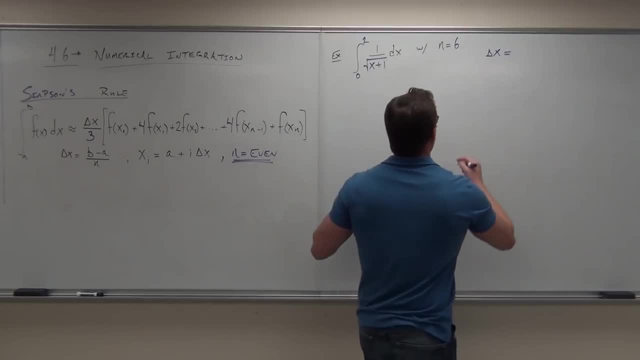 to be satisfying that N is even okay. So delta x, what's delta x? going to be 2 minus 1, 1, 3.. Yeah, it's going to be 1, 3.. 1, 3, that's right. 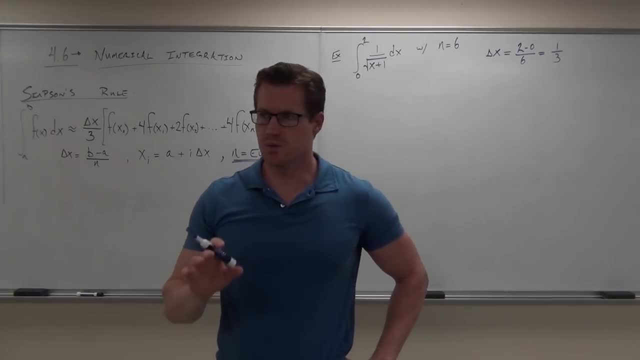 I'd probably leave that as a fraction- 1, 3, because I do not want you to approximate and just do .3 or .33, because you're going to be losing something there and you're essentially going to be losing it every time you multiply. 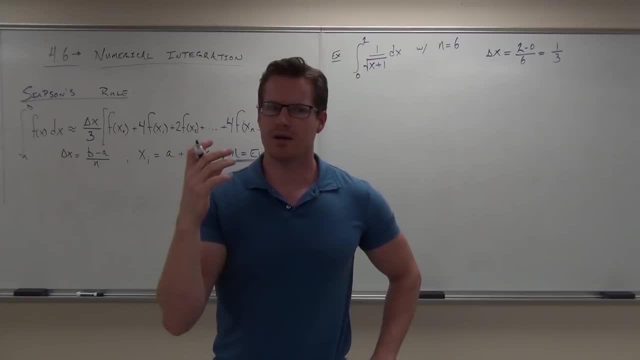 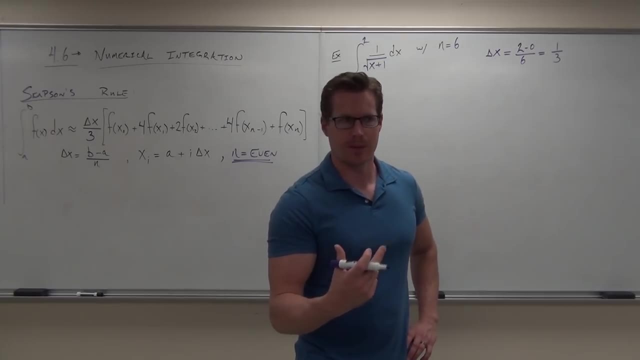 every time you have a term, because of that distributive property, the approximation will be way off. So leave this as a fraction, unless you can have a finite decimal. Are you listening to me right now, Mm-hmm? Okay, so leave it as a fraction. 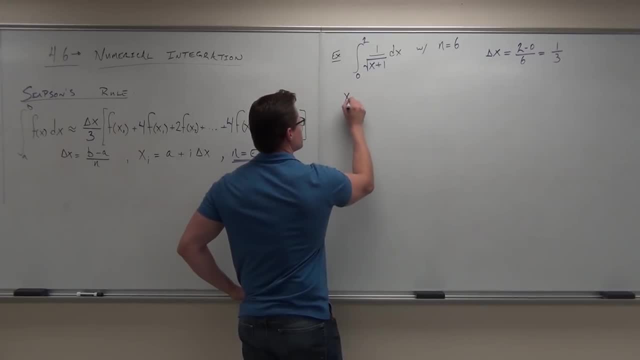 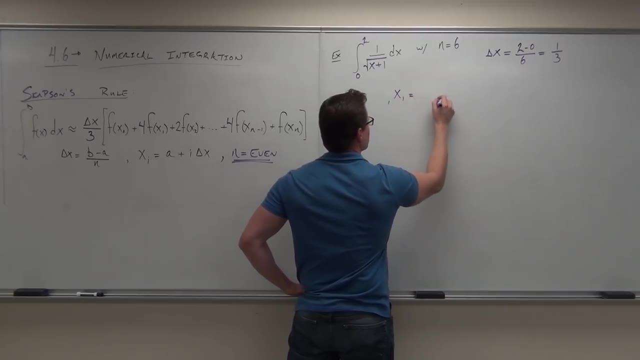 Okay, well cool, Now let's do our x's. So we want x of 0.. We want x of 1, x of 2, and so on. What's x of 0 going to be? Do you know? 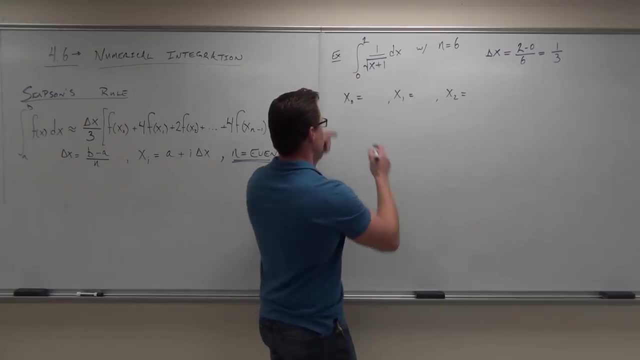 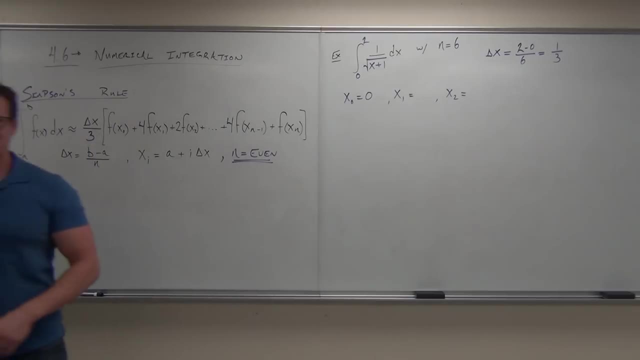 What's x of 0?? Say it louder. What did you say? 0. 0,? yeah, you start with a 0. 0,, no problem, Okay. well now if I have x of 0 is 0,, what's x of 1?? 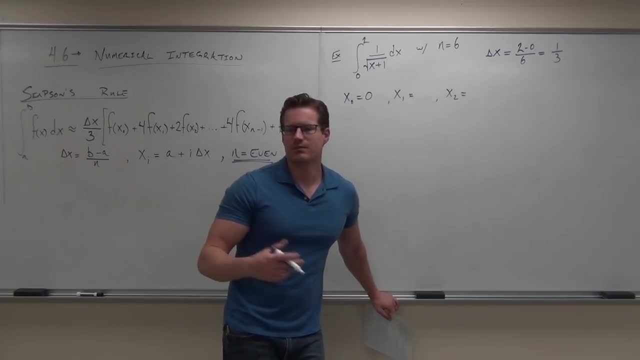 Do you know that? one, 1, 3.. Yeah, it's going to be 1, 3.. Do you guys see the point? Do you guys see the point in doing this? Well, maybe you don't see the point in actually doing this. 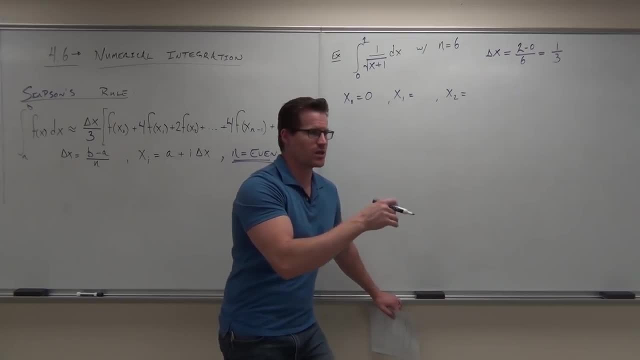 We're trying to approximate integrals without actually doing them. We start with that number. You just keep on adding this, your delta x, for every term. That's what this says. It says: start with your a. Do you understand? our a is 0 right now. 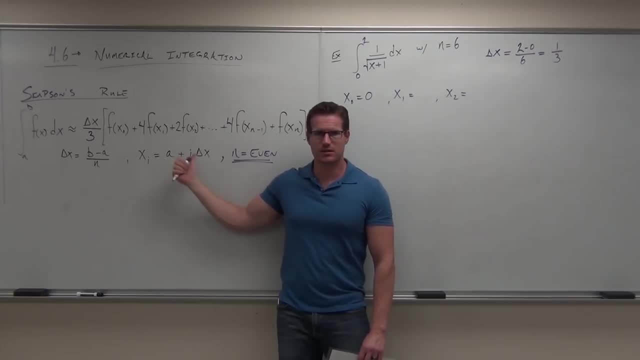 You get it. Start with a. Just add delta x. That's it. Just add it every single time. So what's 0 plus 1, 3? 1, 3.. Okay, we do know how to do fractions. 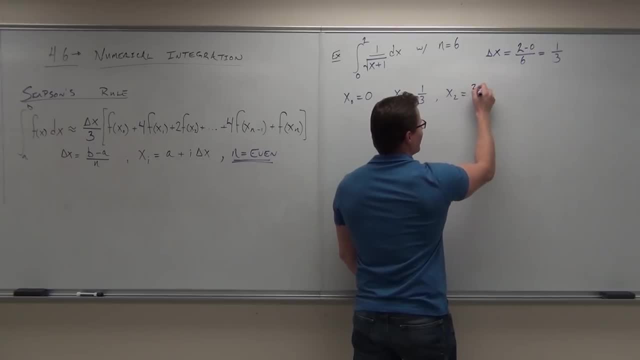 So what's 1, 3 plus 1, 3? 2, 3.. Ah, now we're on a roll x of 3.. What's 2, 3 plus 1, 3? 1.. 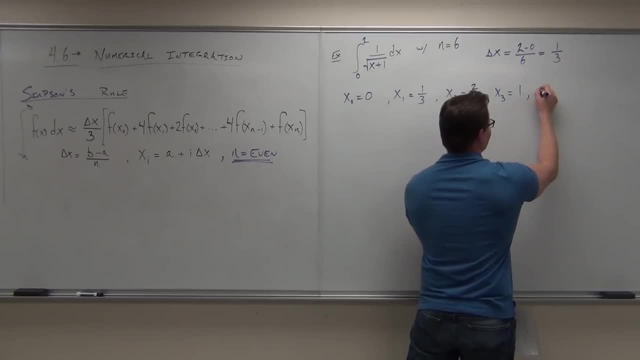 3, 3.. 1. What's x of 4? 4, 3.. 4, 3.. What's x of 5?? 5, 3.. 5, 3.. And what's x of 6?? 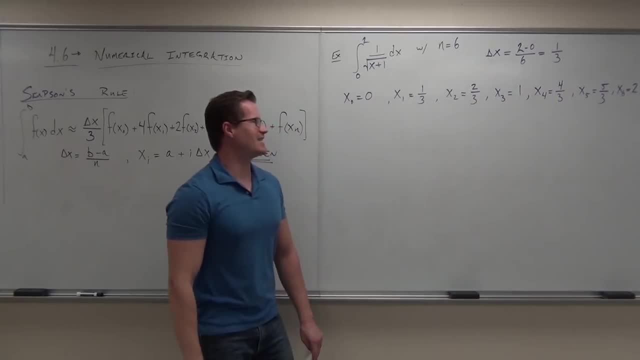 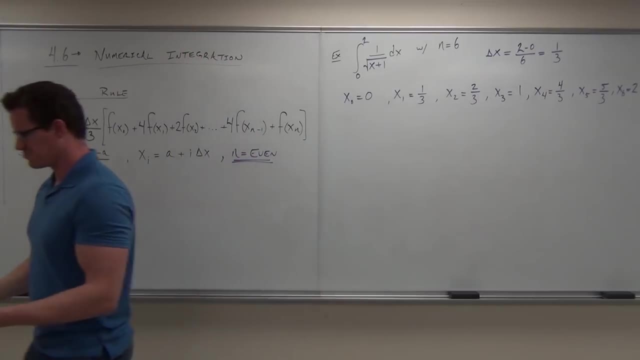 2. 6,, 3. 6,, 3. 2. Yay, So, if any of you are okay with that one, so I have all the terms in this particular one, just so we can go through it and get some time. 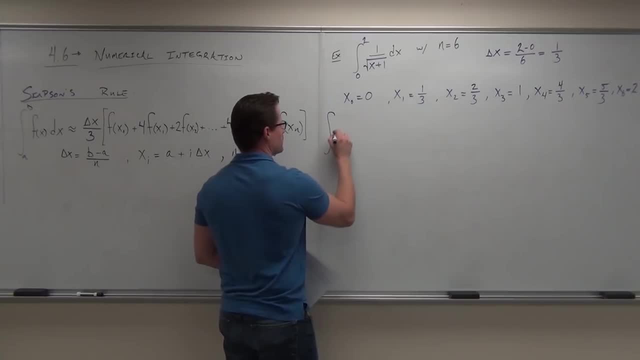 So our integral can be approximated by doing this. We start with delta x. How much is delta x? One third, One third. We divide it by what people? Three, Very good, And then we have this whole sum. We have: 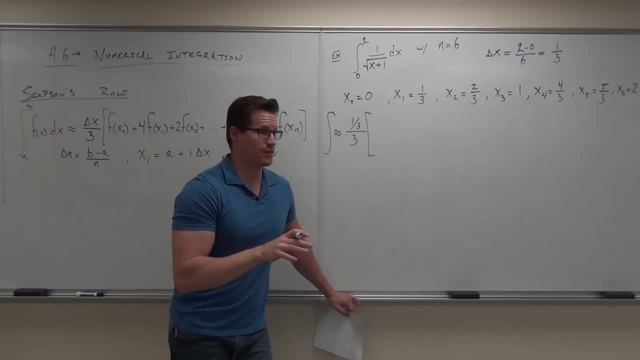 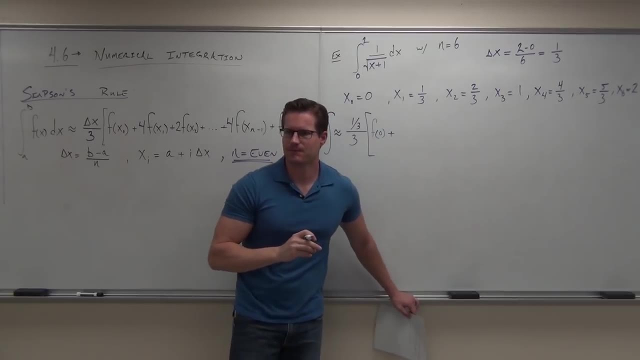 How does it start? F? It leads you to F's, F of 0.. F of 0, very good, F of 0. Then we add: oh, what's the next thing? 4.. 4, it starts with a 4.. 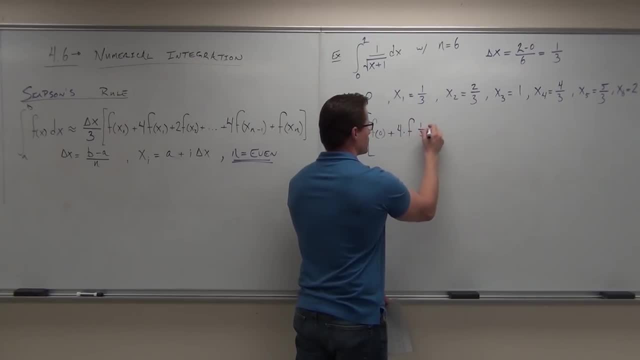 4 times F of what One third One Plus what 2. 2.. Because you go: hey, so it works. Starts with nothing, then it goes 4, then it goes 2.. F of 2 thirds. 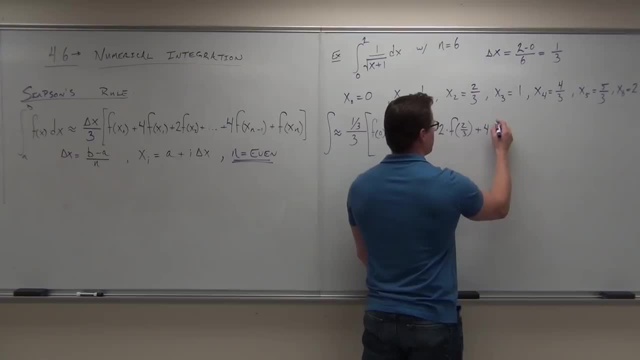 Then it goes to what? 4., 4. Mm-hmm F of 1. 1. Then it goes back to 2. F of 4 thirds. Then it goes back to 4. F of 5 thirds. 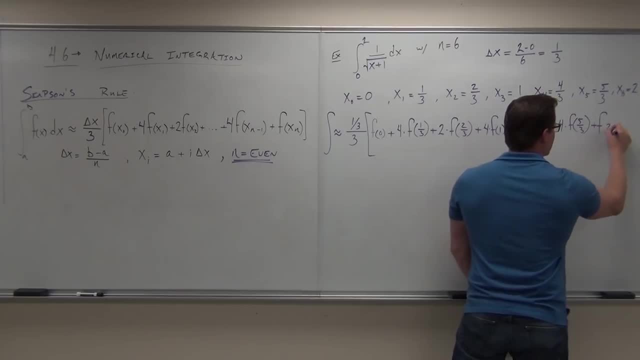 And then it does what please. F of 2., 2. Yeah, But notice there's nothing here. So see how it's going to work. It's going to always start with a 4. Well, start with nothing and with nothing. 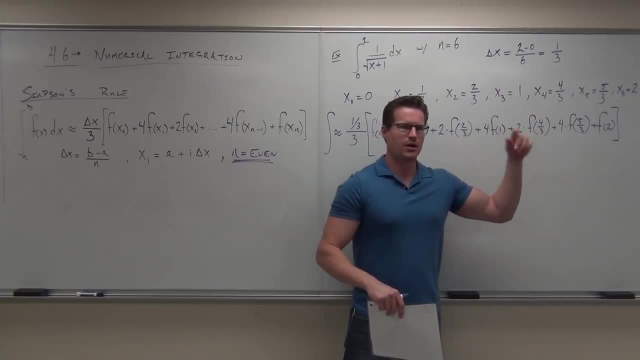 Start with 4 and with a 4.. And we're going to have one extra 4.. So it's going to pair up Bam, bam and then the extra 4.. It's not going to go back to the. it's not going to get there if we use our even ends. 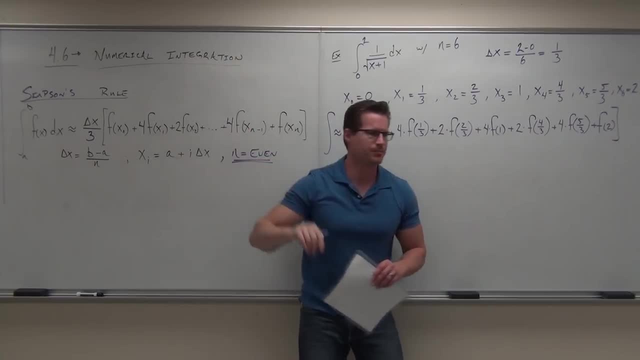 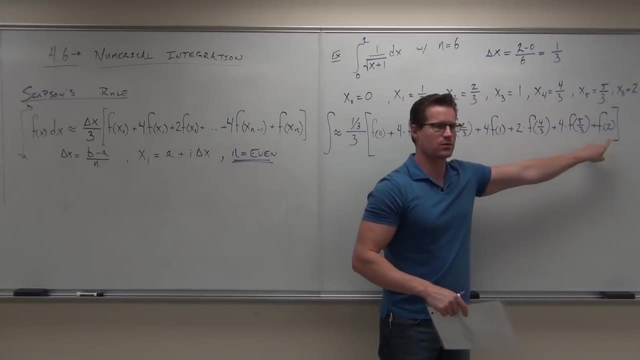 Should I be okay with this one, Are you sure? Okay, And you can see if I went to: n equals 8, what's going to happen is I'm going to have another 2 and another 4.. You see it. 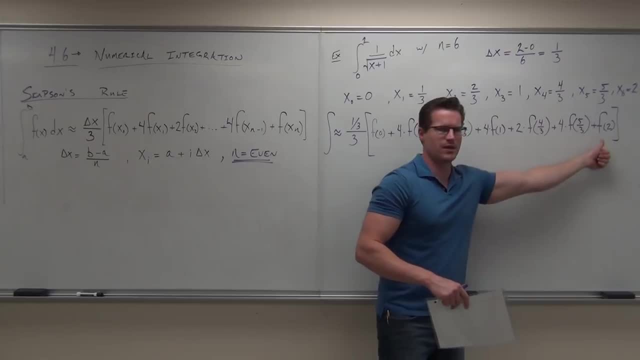 If I went to 10, I'd have another 2 and another 4.. It's always going to end with that 4 and then that last term, without anything in front of it. So what do we do with all these numbers? What do we get to do with them? 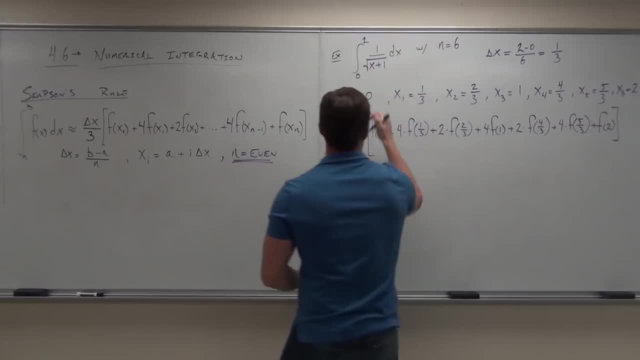 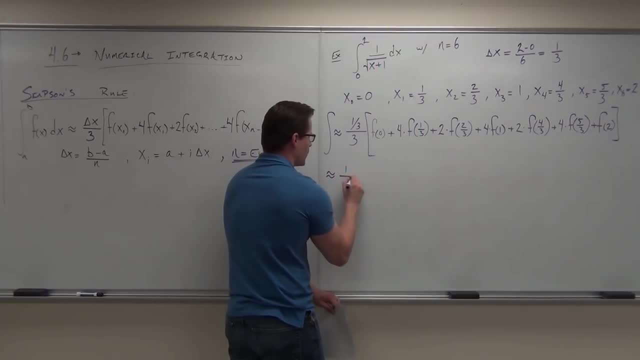 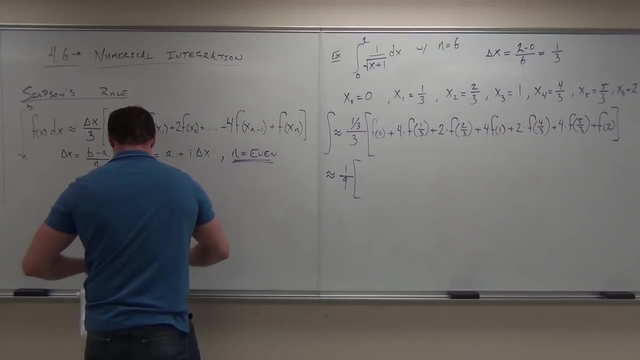 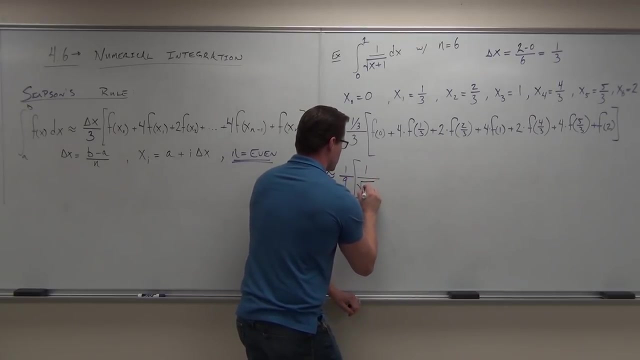 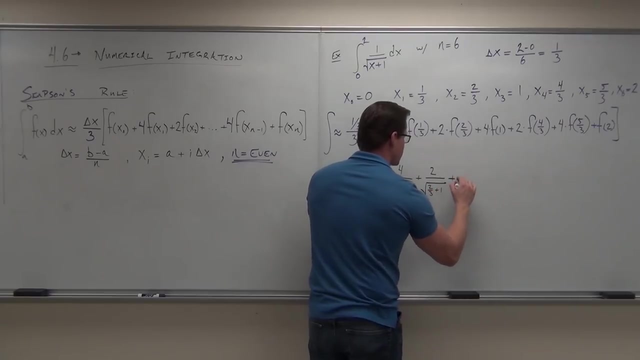 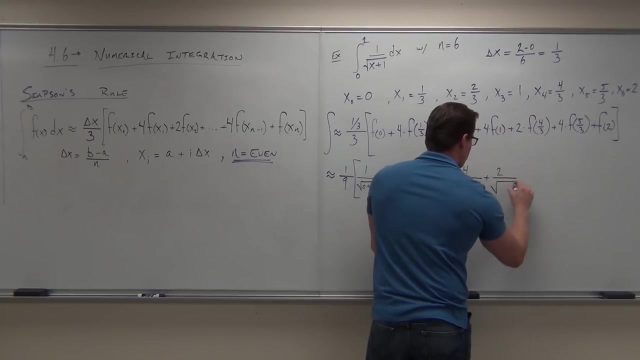 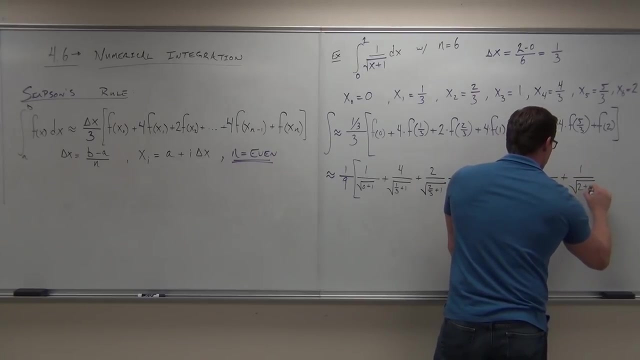 So this is going to be approximately one-ninth. Okay, One over square root, 0 plus 1.. Plus 4 over square root of one-third, plus 1 plus 2 over square root of 2. 3rds plus 1 plus 4 over square root of 1 plus 1 plus 2 over square root, 4, 3rds plus 1 plus 4 over square root, 5, 3rds plus 1 plus nothing, 1, well, not nothing: 1 over square root of 2 plus 1.. 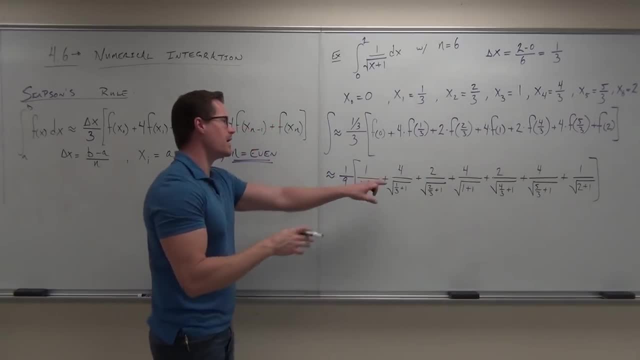 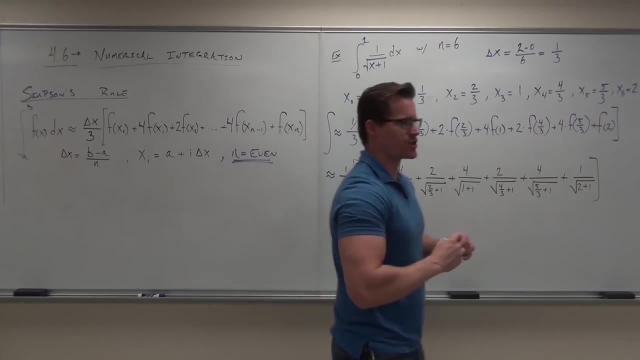 And if you do that and add them all up and then multiply by 1- 9th, then we get an approximation. What I'd like to know is: show of hands if you understand where all these things are coming from. show of hands, if you do. 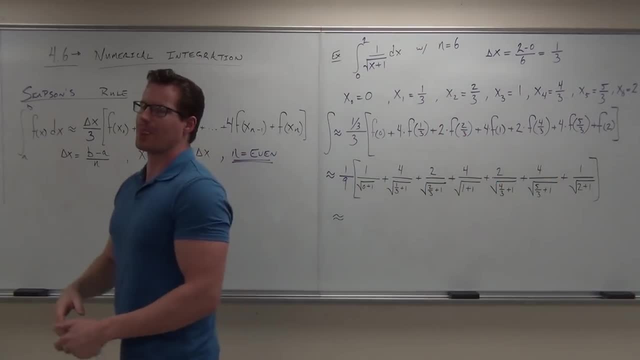 You guys on the right, are you guys okay with this? Okay, so this is why I had to bring your calculator, take your calculators out, because there's a. we're not going to be able to do this in our heads very easily. 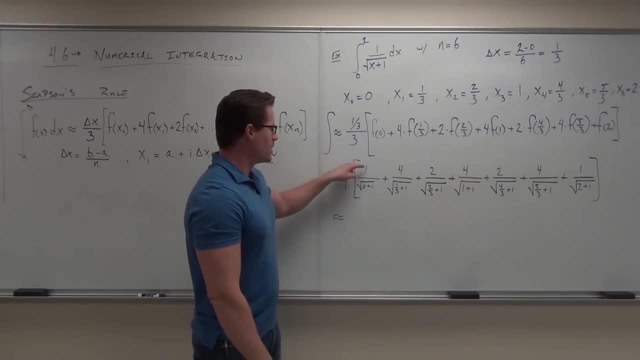 So we're approximating here. it's okay to get our decimals, So we've got 1, then you're going to add that: take a square root, divide 4 by it, and then so on, and so forth, and so on, and so forth. 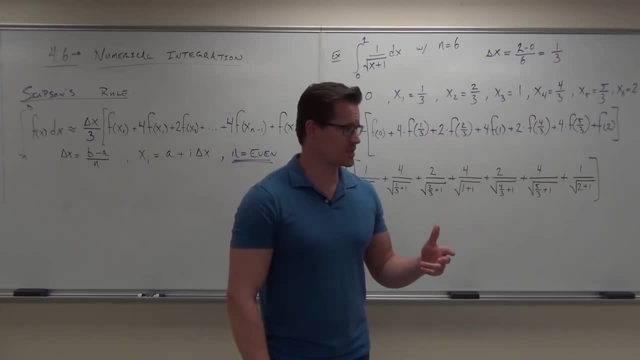 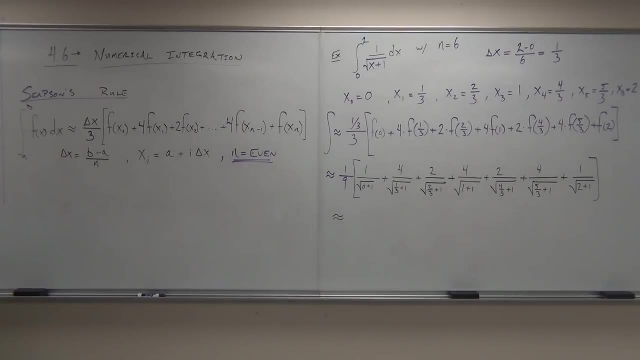 Now I've already done it. you guys can go ahead and see if you can check my work, but just for the sake of time, it's going to take a little while, right? So here's what it is. What it ends up giving you is approximately 1.46421,. is what that is? 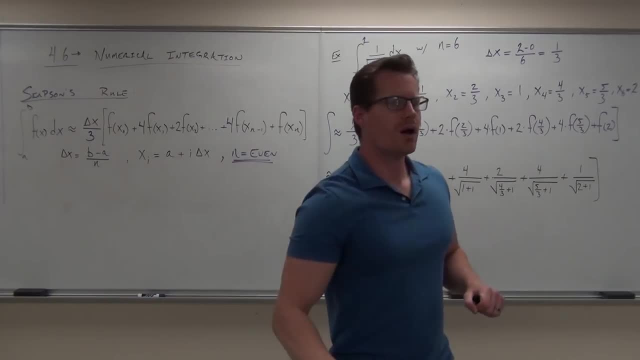 Show of hands if you're okay with the idea. Now what I want you to do is: I want you to do this. What I want to do, I want you guys to do the integral, because we do know how to do this one. 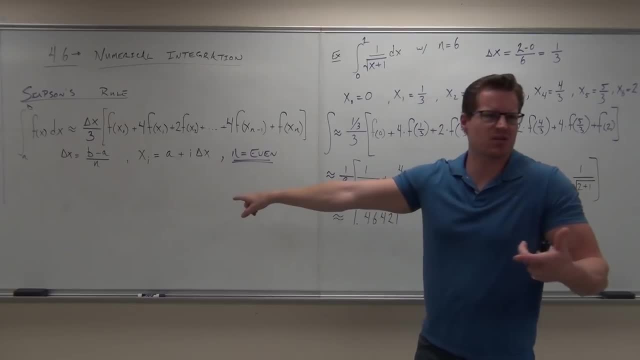 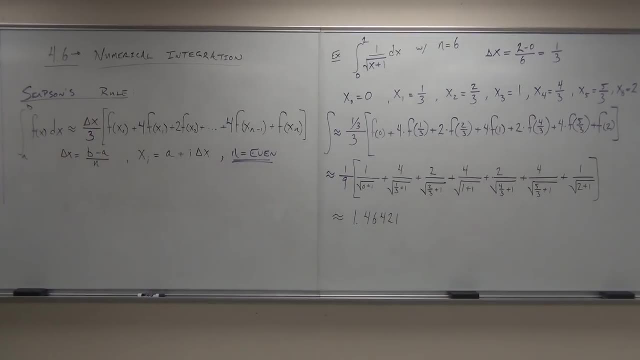 We kind of pretend that we didn't. I want you to do that integral over here and just see how good that approximation is. alright, So go for it. 3., 4., 5., 6., 7.. 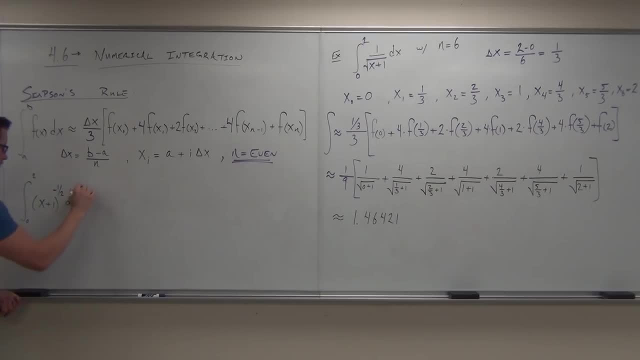 8., 9. 10. 11. Check, 14. 15. 16. 17.. Thank you, I'd like you to check my work to make sure that we all got the same thing. Did you get about that? 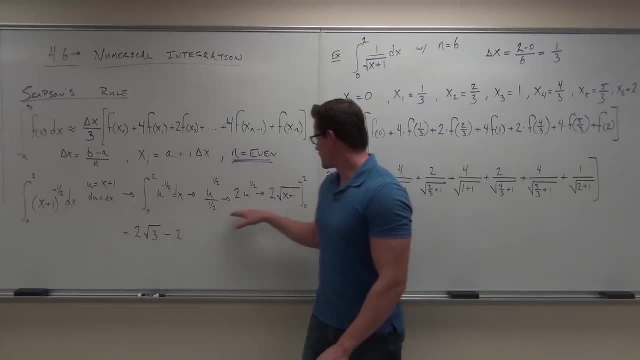 I should just get exactly that. You should know. You got the 2 square root of x plus 1.. Did you plug back in the x before you started evaluating? Perfect, That's fantastic. So we got 2 root 3 minus 2.. 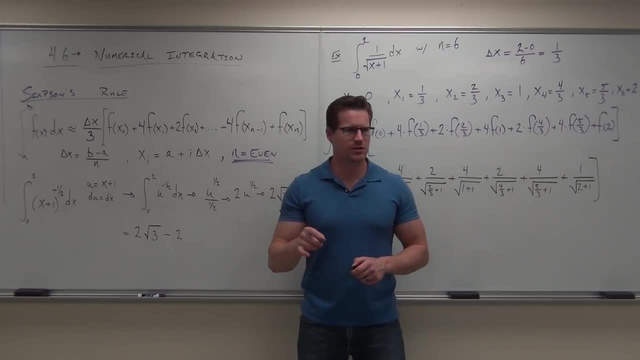 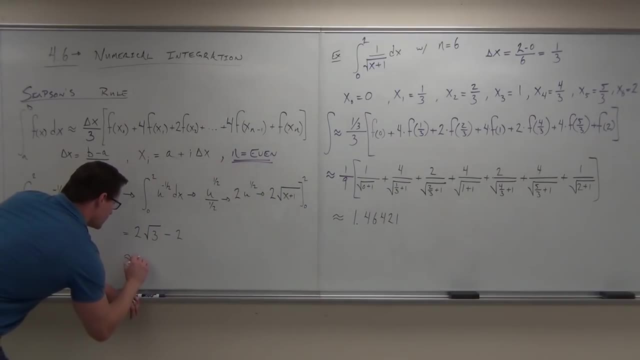 How much is 2 times the square root of 3?? 2 times the square root of 3 minus 2.. 1.464101.. Can you say it one more time? 1.464101.. Okay, that's good enough. 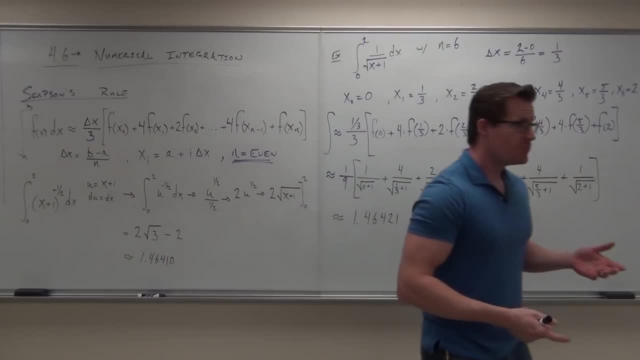 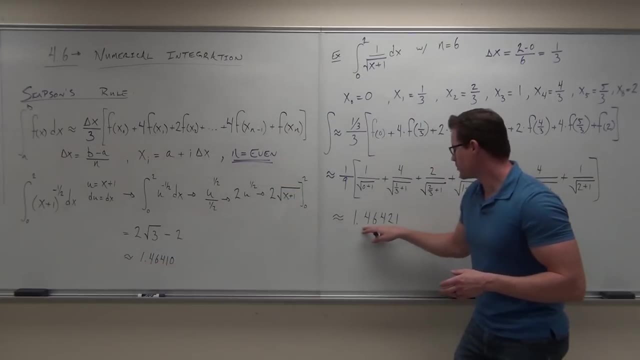 That's our decimal place. Is it exactly the same? Is it close? Yeah, It's really stinking close. Look at that. This is 1.4641.. This is 1.4642.. It's off by 11.. 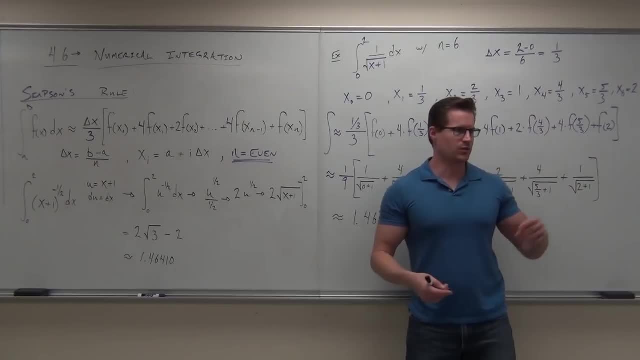 Little over 1 ten thousandth after only 6, ending with 6.. So 6 iterations, That's not too bad. So that's pretty darn close for approximating something if we didn't know how to do it. So that's how the trapezoidal rule works.